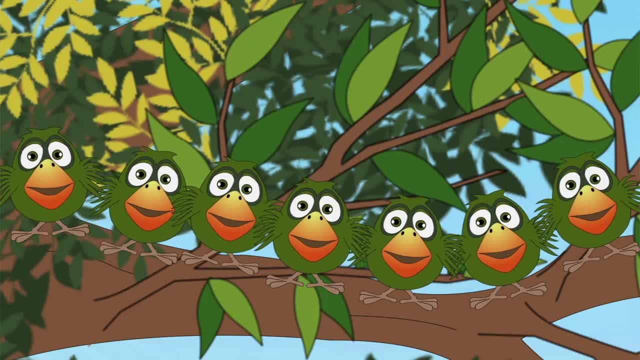 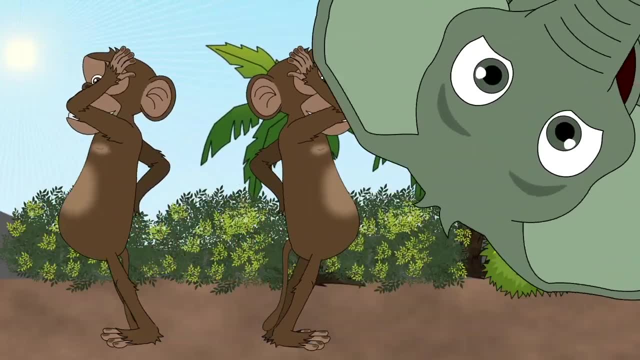 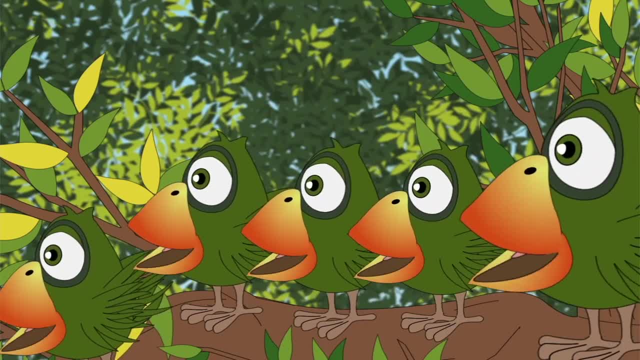 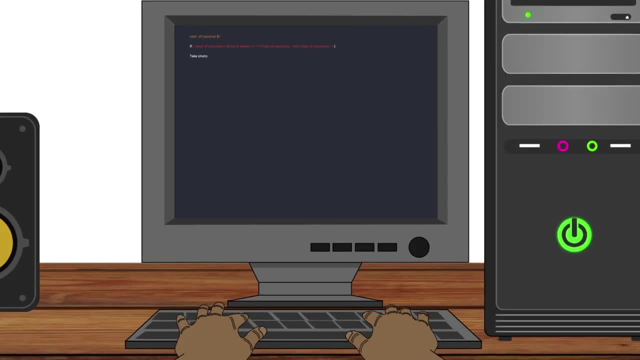 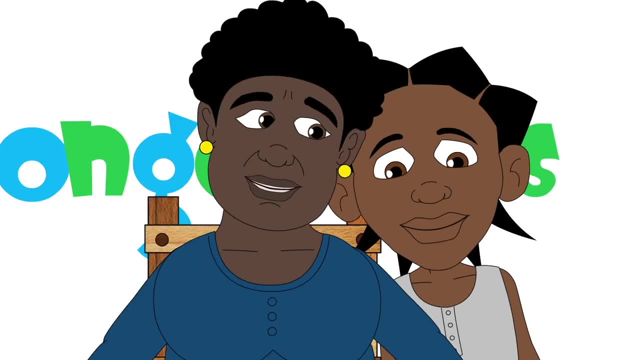 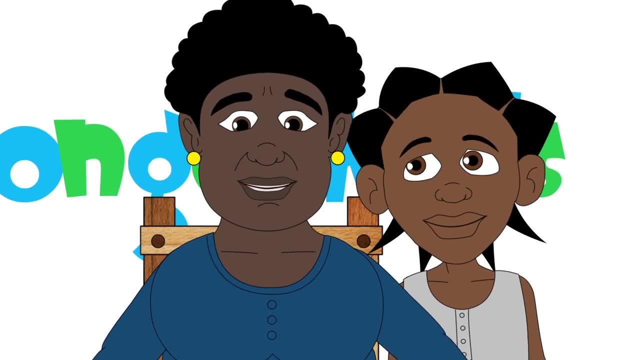 And what are all those strange words you're writing? I'm talking to my computer. Um, I don't think you can talk Mama Tech, Not like we're talking now, but I can communicate with it. I'm talking to the computer by coding Kibena. 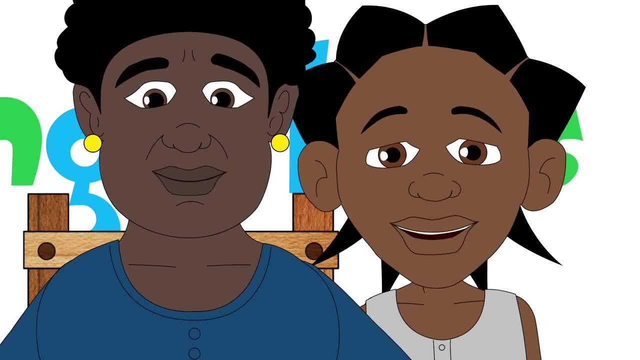 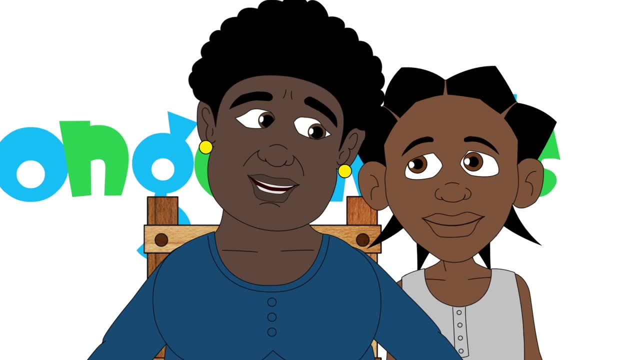 Coding. Is that those funny words? I can't understand. well, any of it. You must be a genius, Mama Tech. You don't have to be a genius to learn code, You just need an open mind and a little bit of practice. 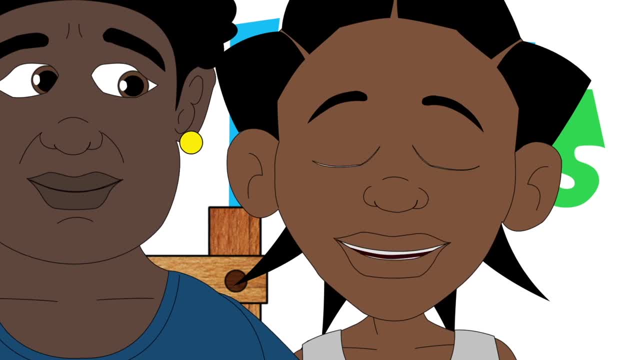 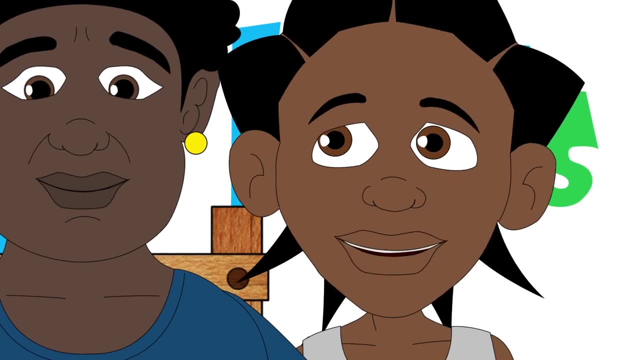 Then anyone can talk to computers. No way You think anyone can learn that? I've only used a computer once. No way could I talk to one. You don't even need a computer to learn code Kibena. All you need is your Ubongo. 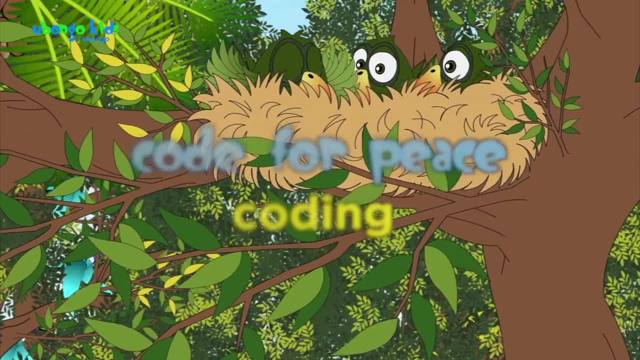 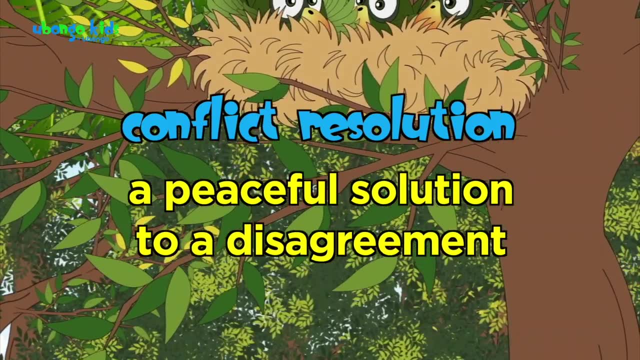 I guess I said I'm a genius. How do you think I can learn a lot? I'm a genius, Kibena. You've got to be a genius. I've got to be a genius- What? I'm a genius too. 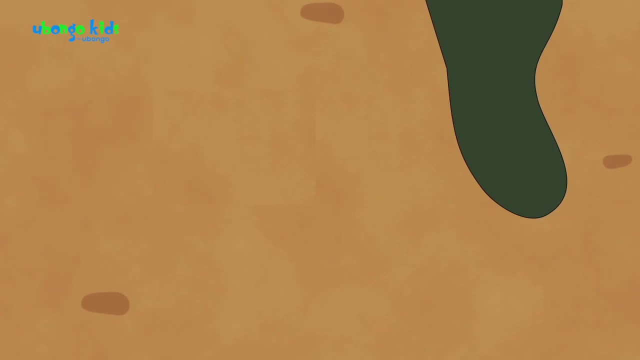 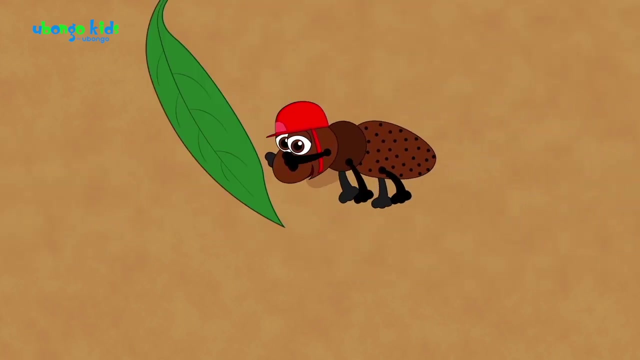 I already are a genius. I'm just a genius. Hey, Kibena, who theцию? Hey, what's wrong? What did you say you were doing? I'm a genius. I'm an artist. I'm a genius. 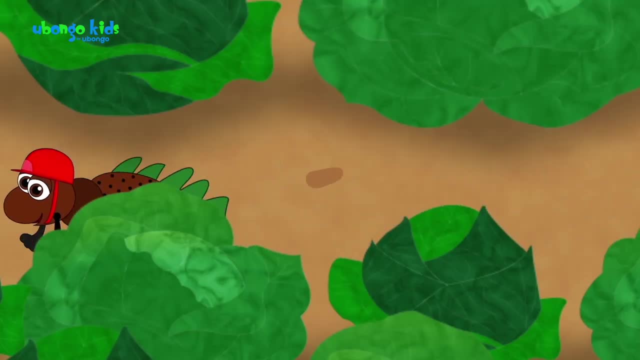 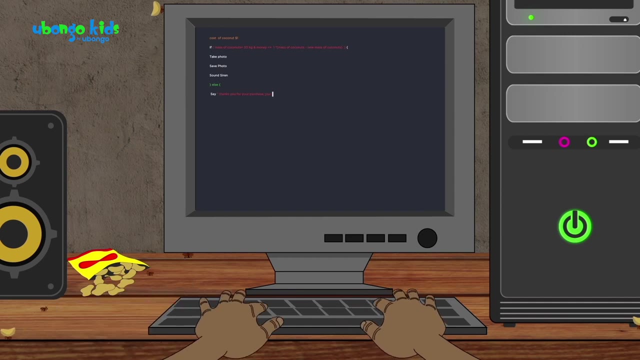 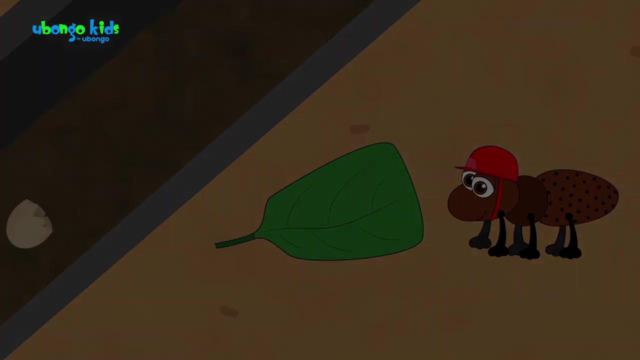 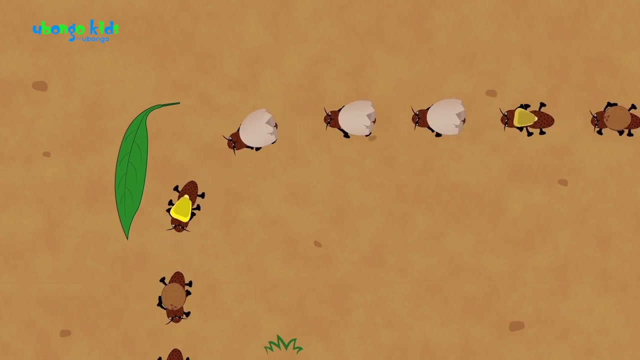 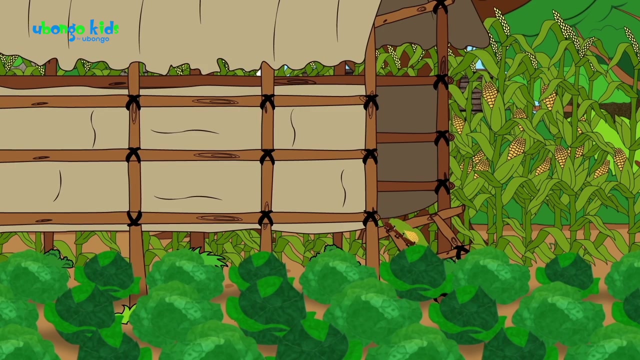 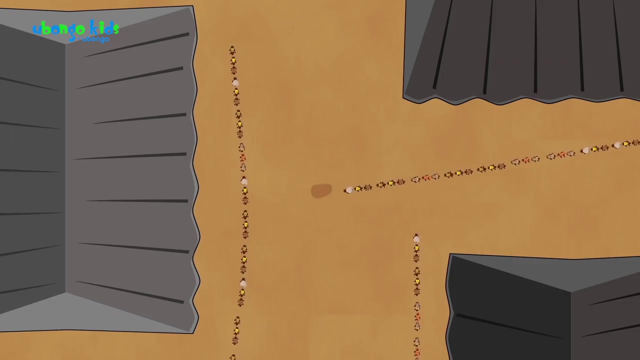 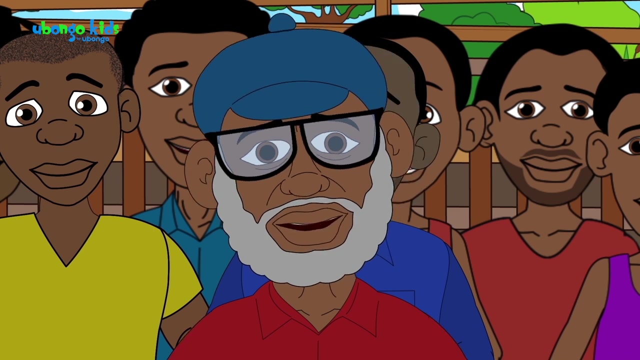 Hey, you are a genius. Hey, I have had it with these ants. They're everywhere. You know, over half of my coconuts were ruined. today I came home to find my rice bag completely empty. Ugh, those ants. 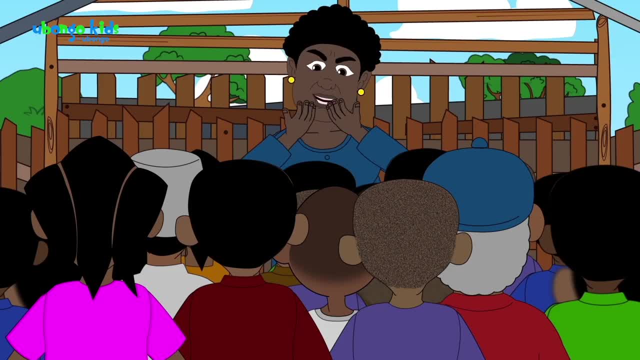 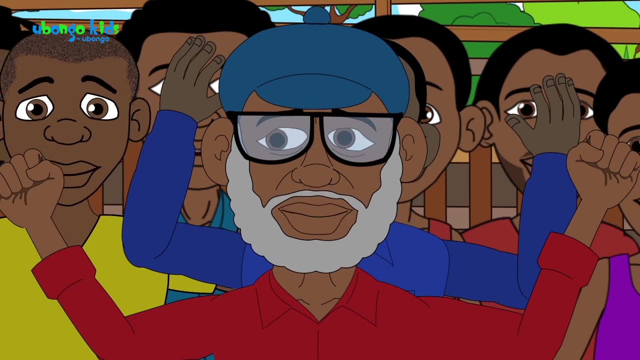 Hey, they even attacked my DVDs. That's it. It's time to fight back. We will fight back. So it's time to fight back. Let's fight No peace, peace, I I mean there's no need for fighting. 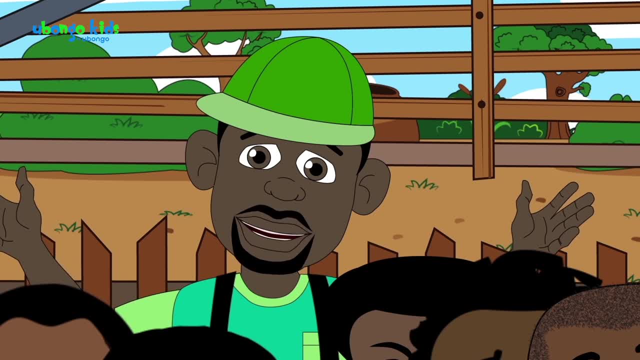 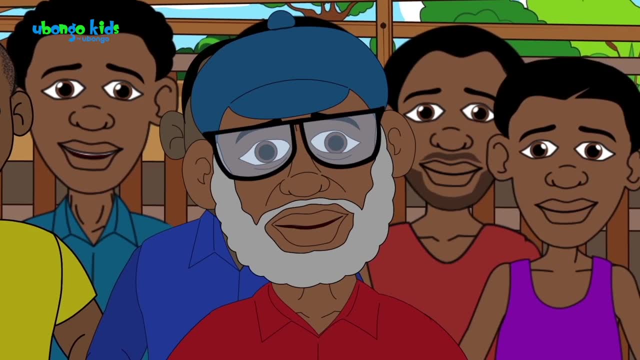 The ants just need food to eat. There is no way they can eat as much as they're taking Those greedy little rascals. They are thieves, they are Ugh. they take more than they need. A year's worth of rice for a human they took. 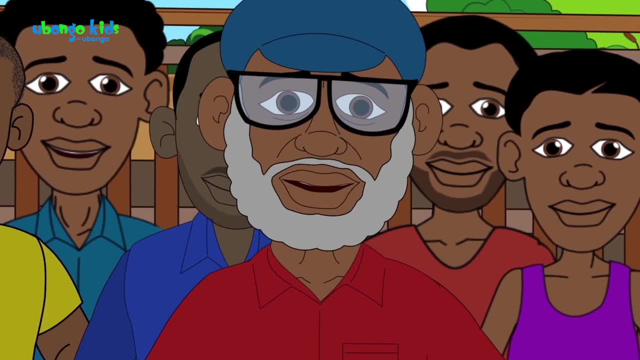 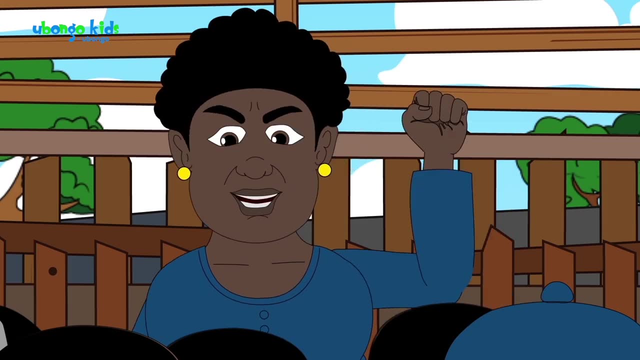 That will last them a decade. I've had it, So it's time to fight. Let's get out the spray. The spray, Please, Mama Tech, everyone calm down. We need to at least try to solve it peacefully first. 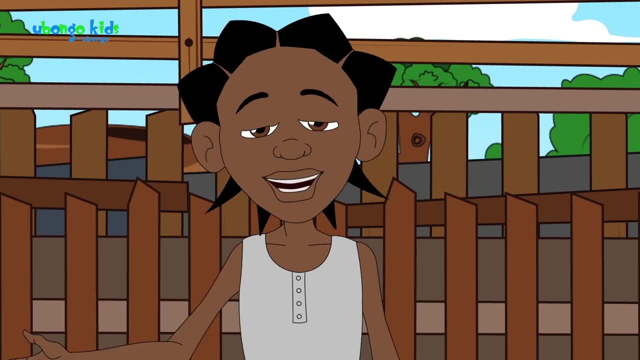 I'm sure we can find a solution that would work for everyone. Please, let's all just calm down, Take a deep breath. Once we're calm, we can start to understand each other. The famous scientist, Einstein, Einstein, Einstein, Einstein. 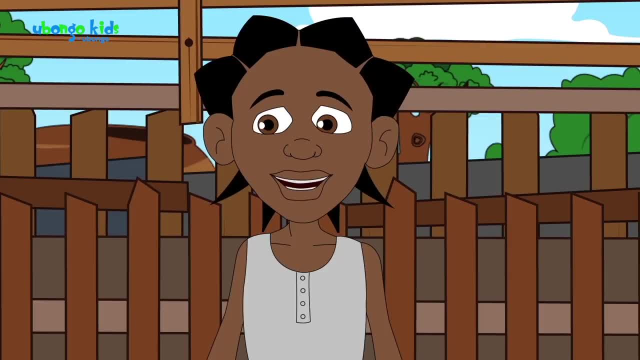 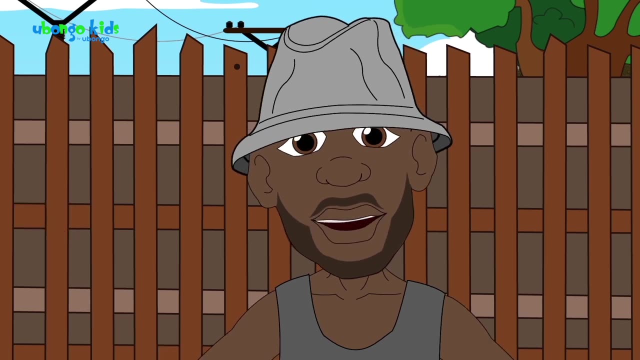 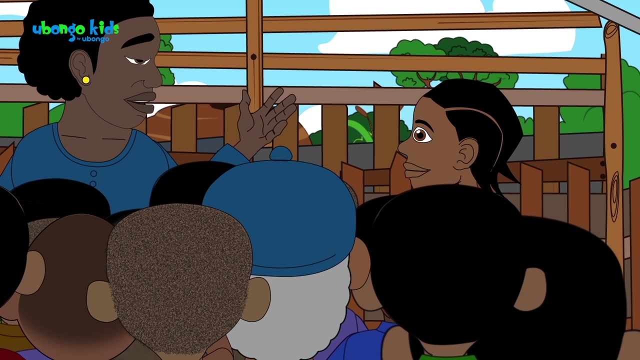 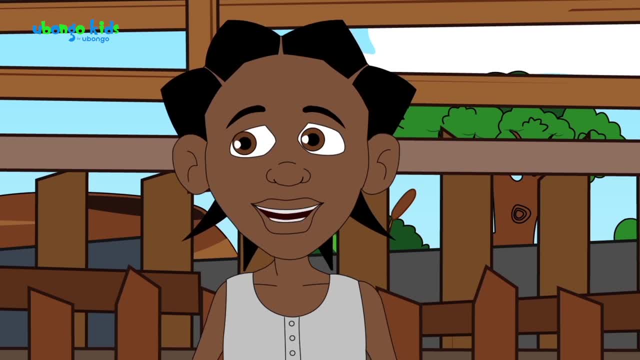 Einstein. Okay, Xibena, we'll give you one day, But if you haven't solved this peacefully, based on tomorrow morning, we are going to fight those sands. Whew, okay, Hey, That was amazing, Xibena, You were really brave. 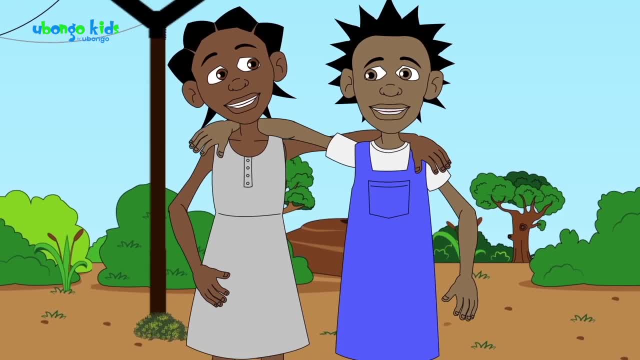 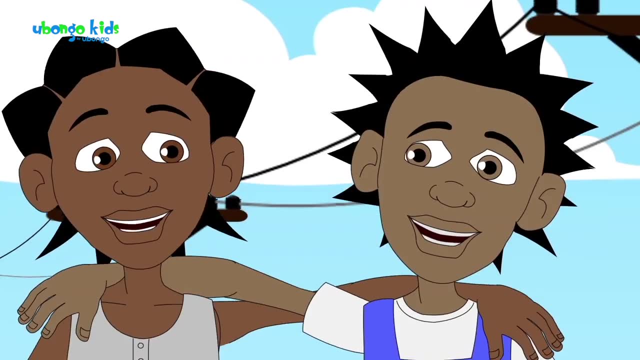 I don't feel brave. What are we going to do now? We only have one day to sort this mess. Not sure, but it seems that we have the beavers- Maybe the best thing we can expect, But they're more types than we thought. 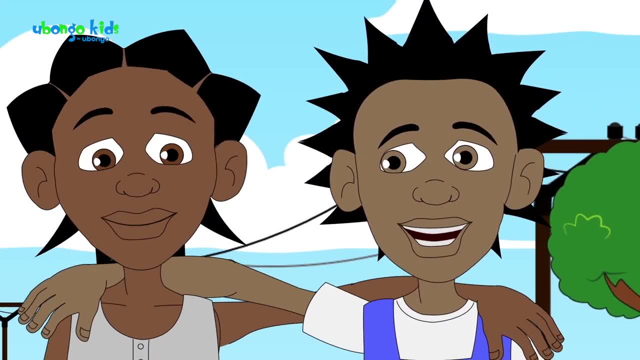 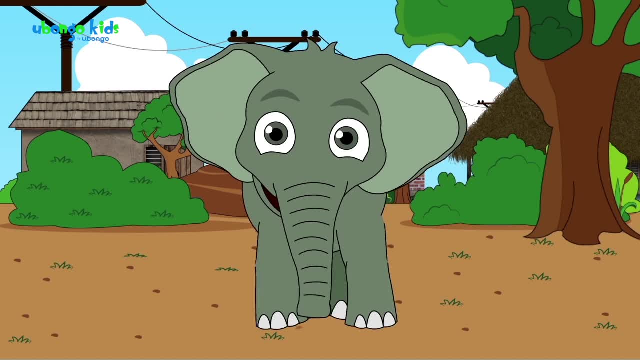 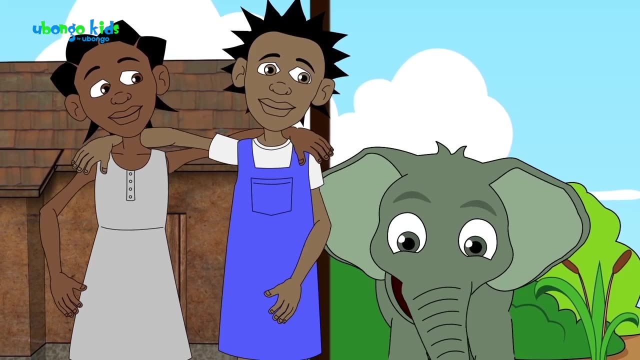 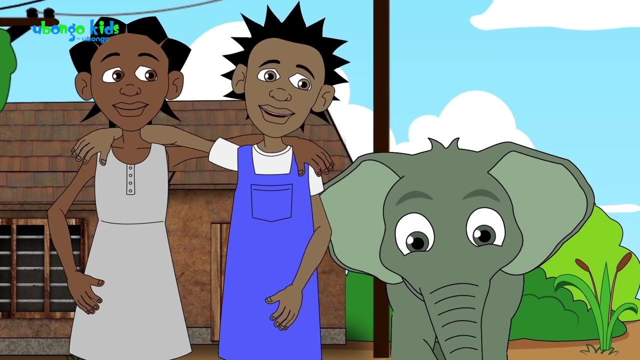 Not sure, but I think I know who might be able to help Tembo Tiny Tembo, Tembo Tiny Tembo. What's the problem, friends? Kibena, the peacemaker here, has 24 hours to get the ants to stop taking people's food and crops. 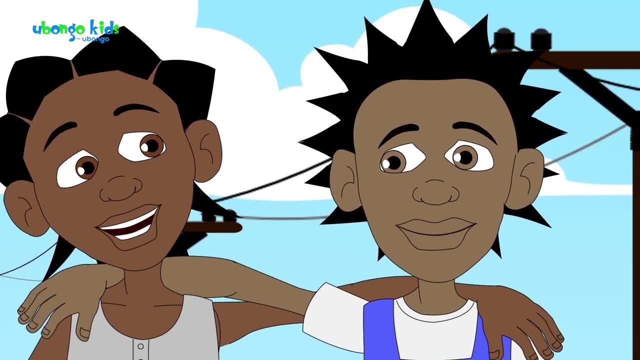 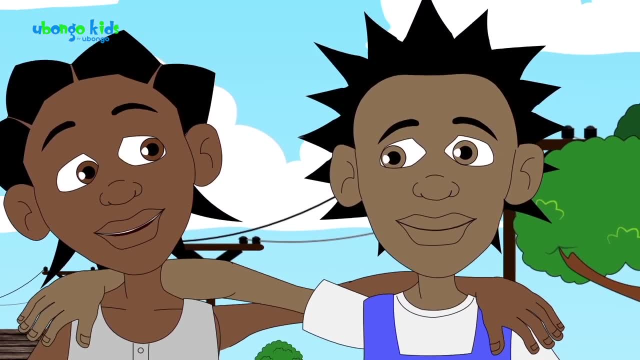 The next step to conflict resolution is understanding both sides' point of view. The people have already made their views heard. Now it's time we talk to the ants. We need to know why they're taking so much food. Oh, I love chatting with insects. 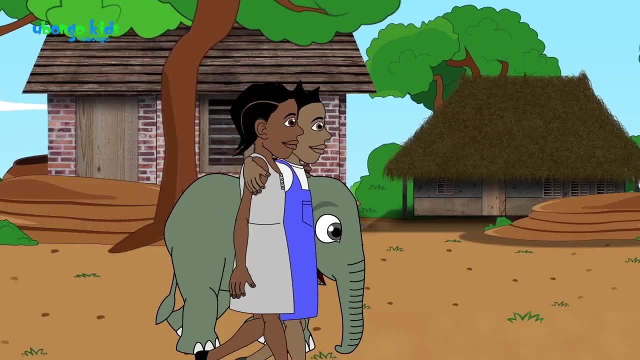 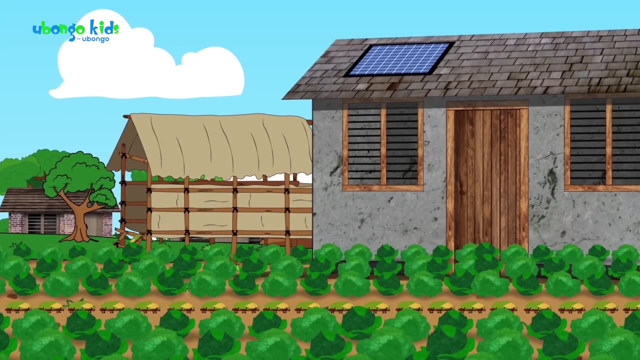 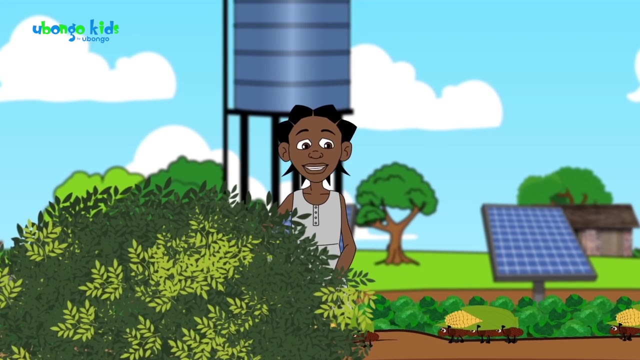 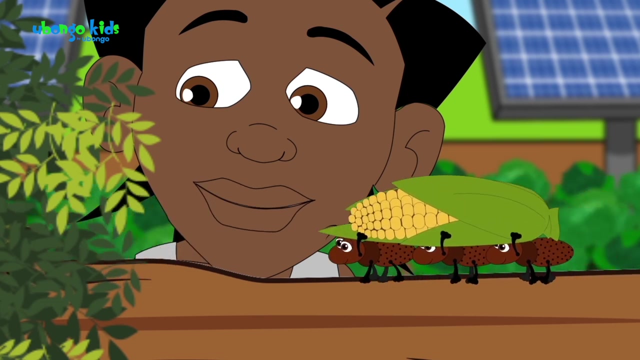 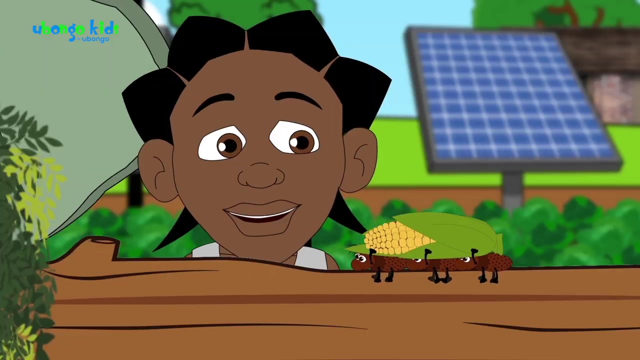 I had a fascinating conversation with a termite once. You can't imagine the intricacies. Ahem, Um, excuse me, Ms Ant. Oh you, Ms Ant, Could I bother you for a? We'd just please like to know why you're taking so much food. 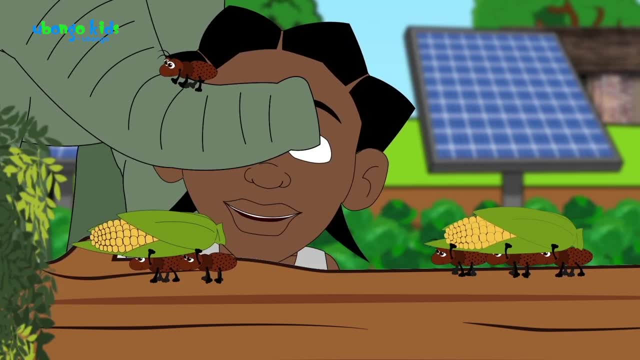 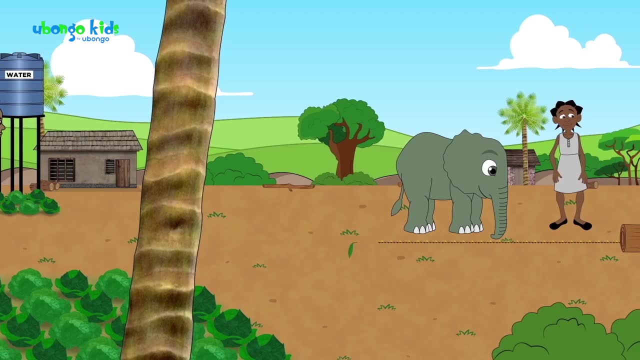 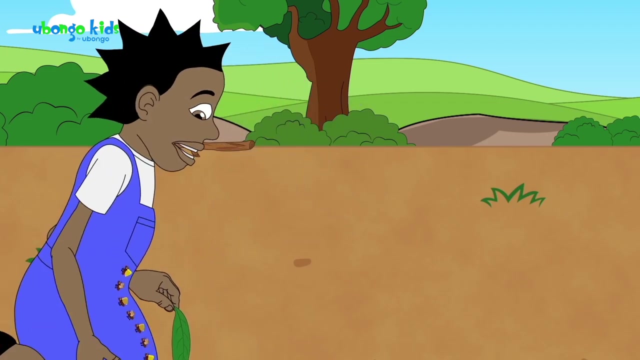 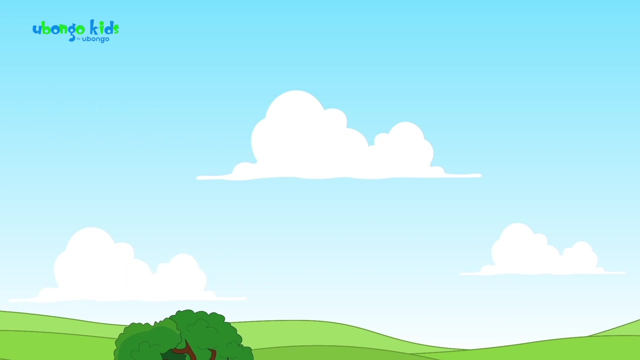 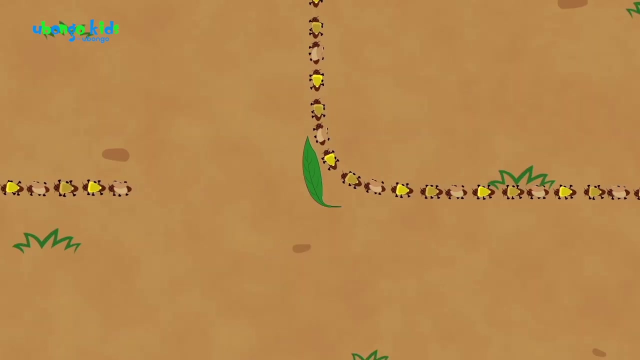 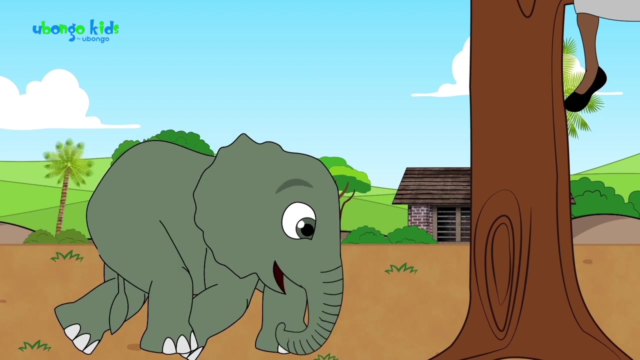 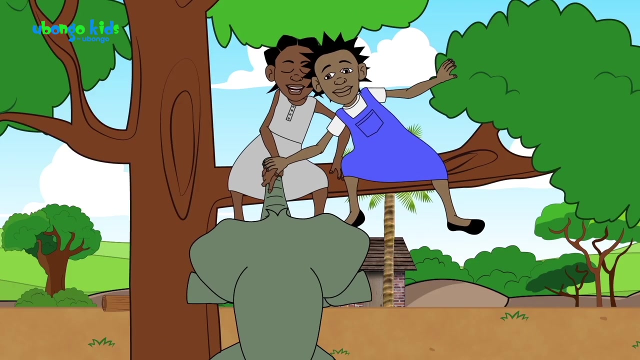 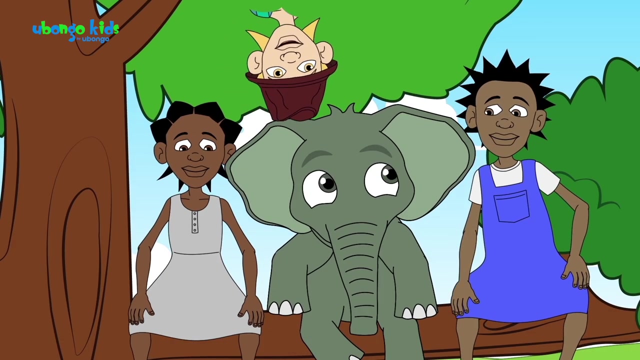 It's more than you could possibly eat yourselves, and well, we No. There must be another way that they communicate. Ah, Quick Up the tree. Now. I don't know what's more strange: elephant climbing a tree or the behavior of those ants. 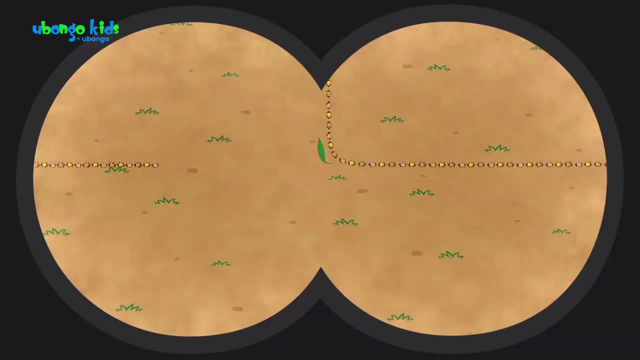 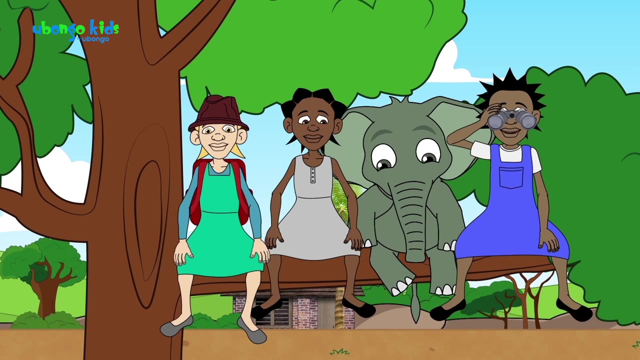 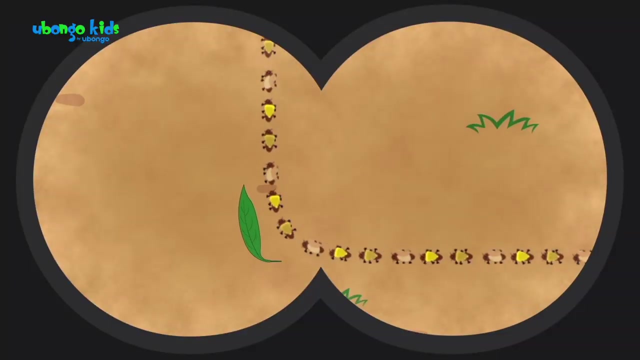 down there. It's something to do with those leaves. Huh, look, all the ants are turning at the leaf And since I flipped the leaf, they're going in the opposite direction from before. Look, they're all stopping over there. 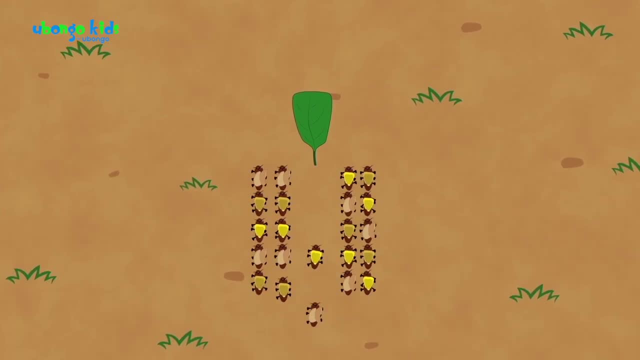 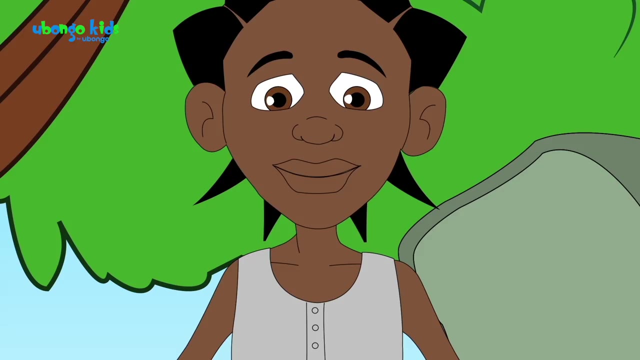 I'll bet you it's because of the leaf. That must be how they communicate. So the question is: how can we use the leaves to communicate with them? We still haven't answered our first question: Why are they taking the leaves? Why are they taking so much food? 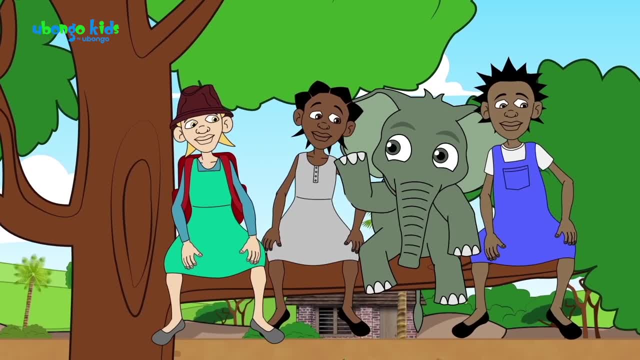 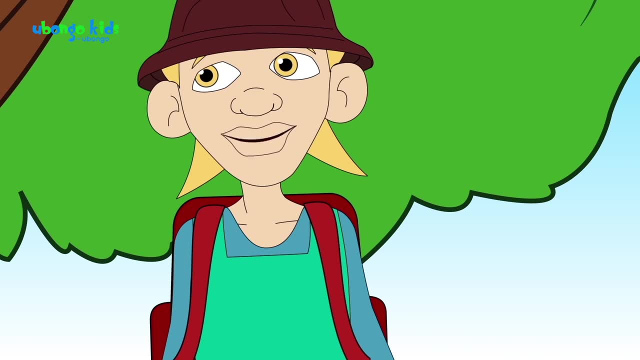 And even if you answered those two questions, I've got a third for you. Where are we going to tell them to go instead? The first step to problem solving is asking the right questions. Now it's time to go and find the answers. 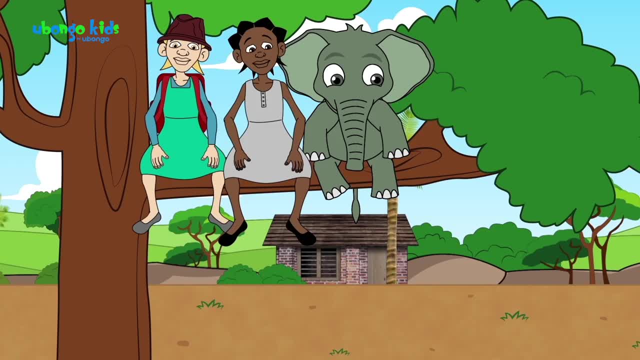 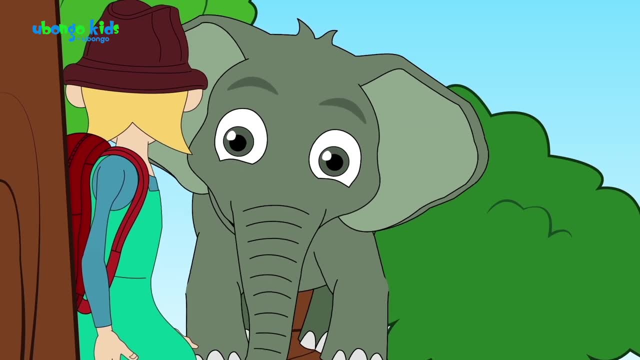 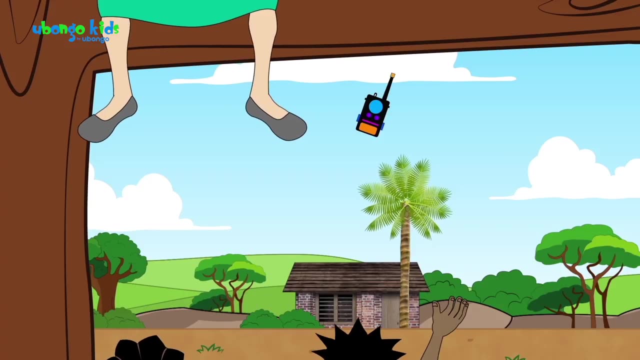 I'll find out more about how they use the leaves. I'll follow them to figure out what they're doing with the food and why they need so much Steady there. Tiny Tambo and I will stay here to observe and document Hm. 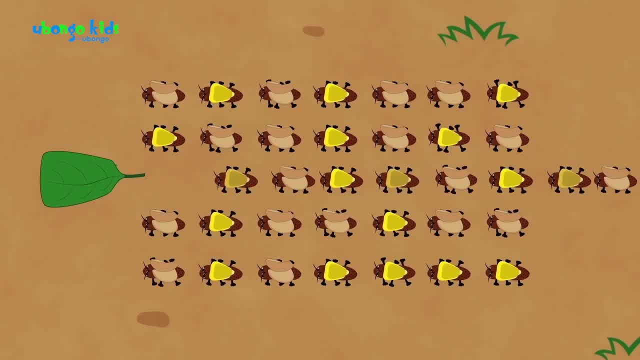 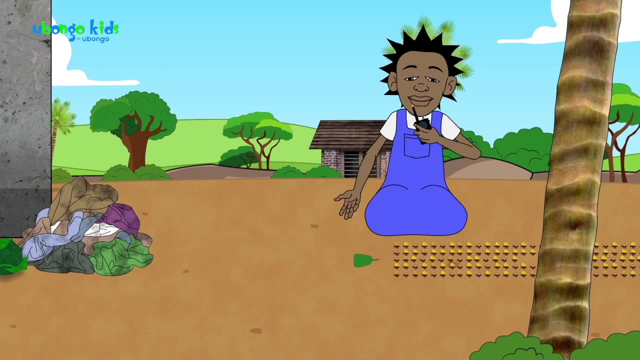 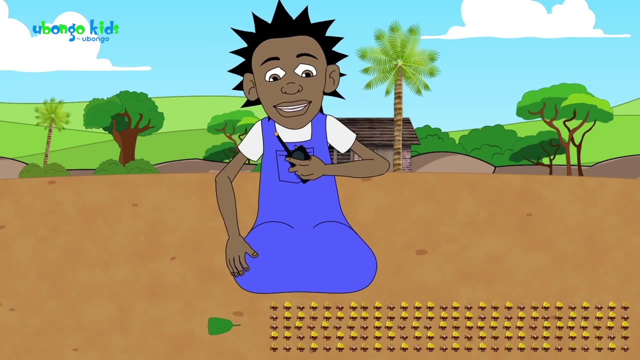 They're all stopping in the same spot. at this leaf It's kind of round with a flat bit at the top. I've got an idea of what this leaf does, But I'm going to test it out to make sure Let's go. 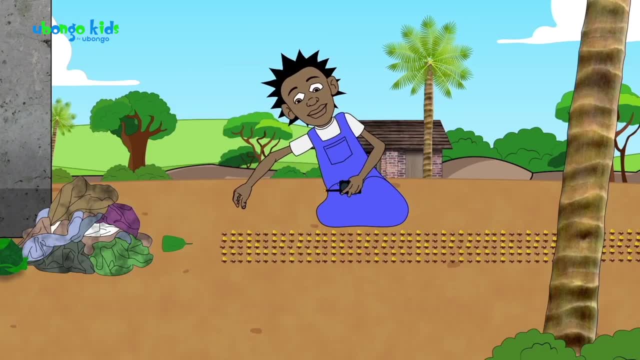 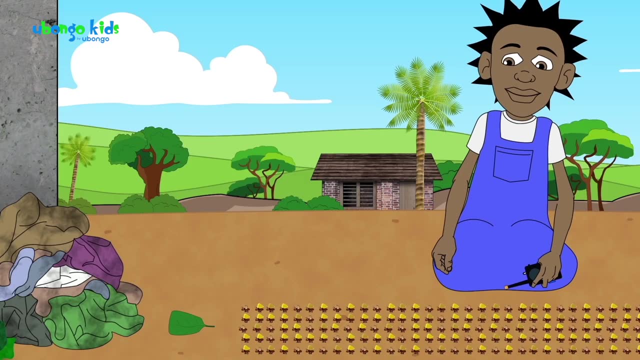 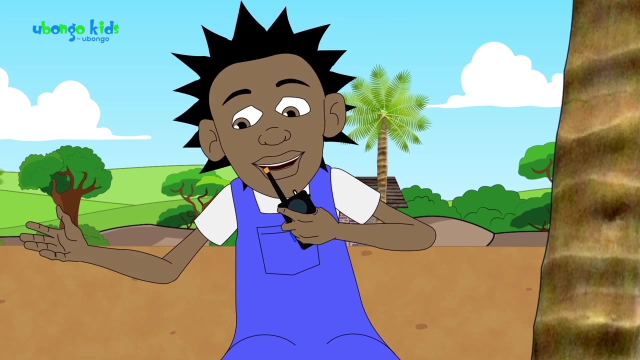 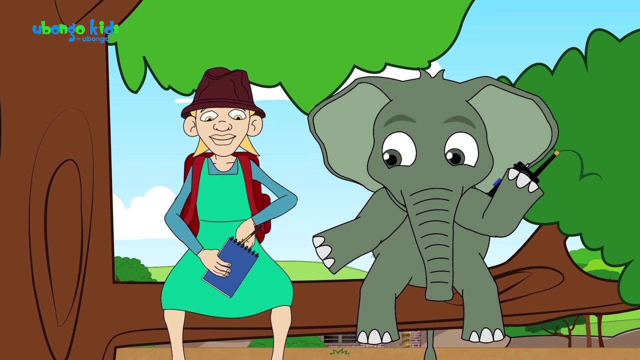 Phew Zekiko would have had ants in his pants. Kiduchu to Tiny Tambo. It's confirmed. The flat-topped leaves mean stop. Copy that Flat-topped leaves mean stop. OK. Curved leaf means turn and flat-topped leaf means stop. 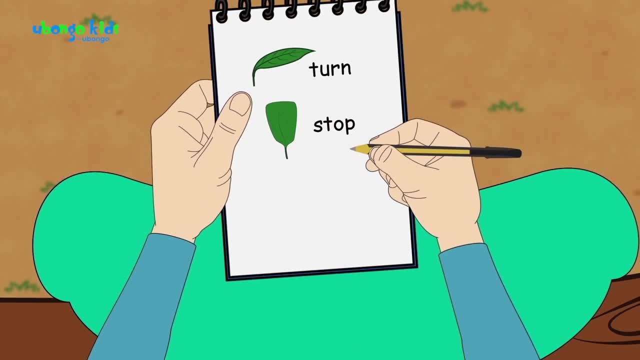 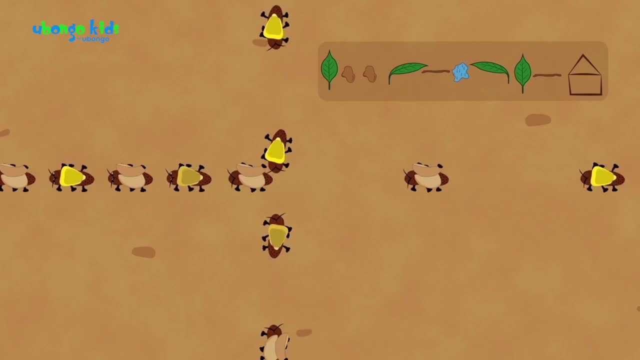 Got it. Now let's check how Kibana's doing. Titi to Kibana, Titi to Kibana, Hi, Titi. I'm still following the ants. There's a spot here in the forest where all the different lines of ants are coming together as one. 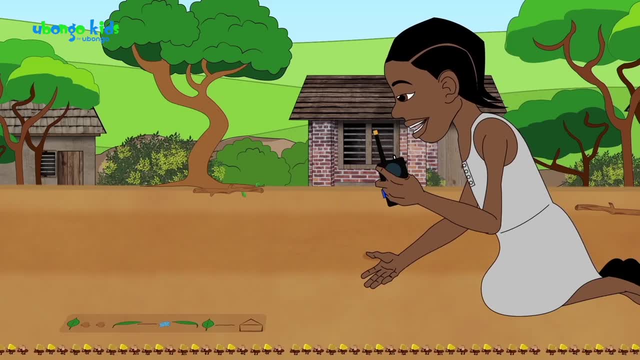 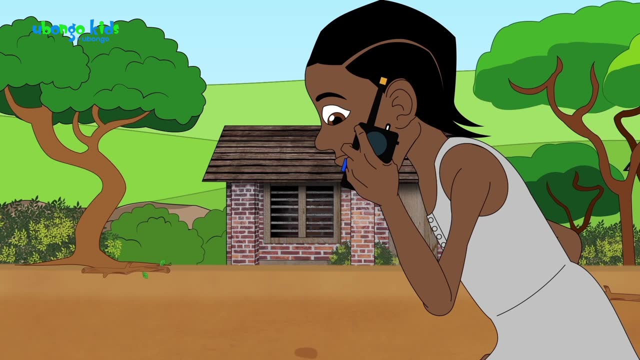 And there's a whole bunch of leaves here, along with rocks and sticks and drawings too. It's like a maze, It's like some kind of code Code. What's a code, Kibana? A code is a system of communicating through symbols. 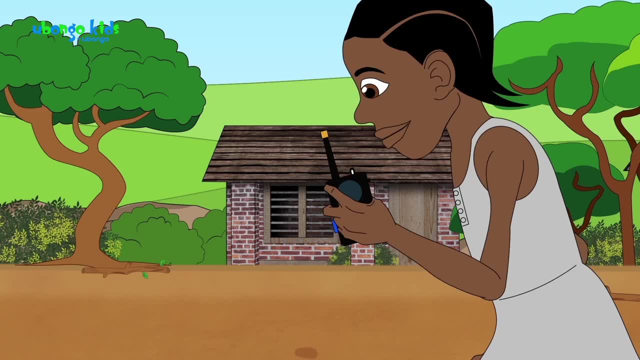 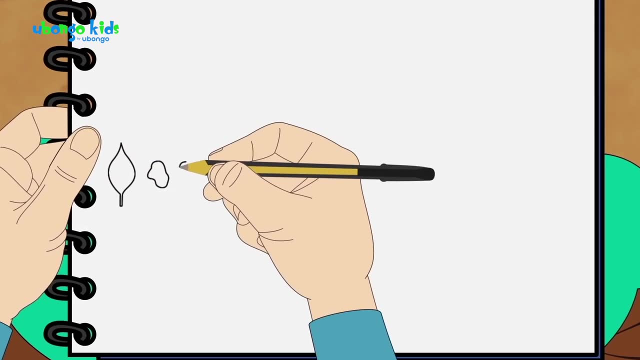 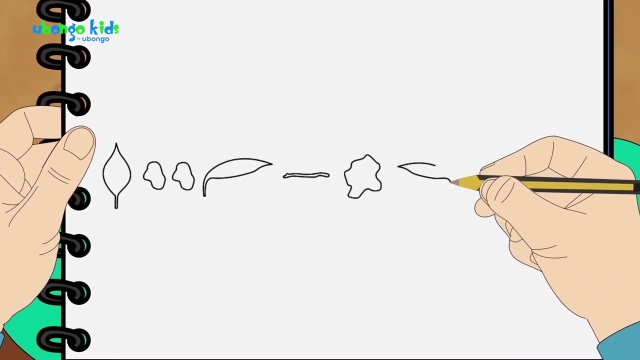 And man, this ant code is complicated. Read it out and I'll record the code. OK, Pointy leaf- two rocks. leaf curve to the right, long stick, a drawing of a pond. a leaf curve to the left, a triangle-shaped leaf- another long stick. 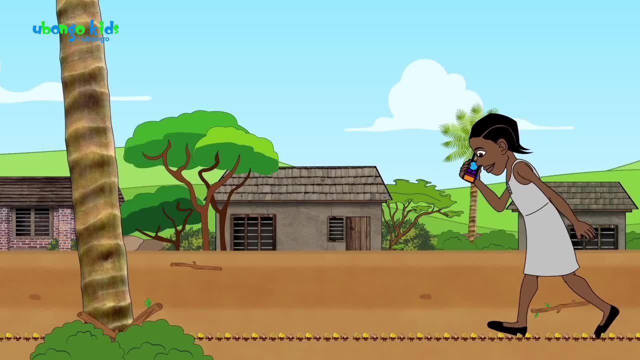 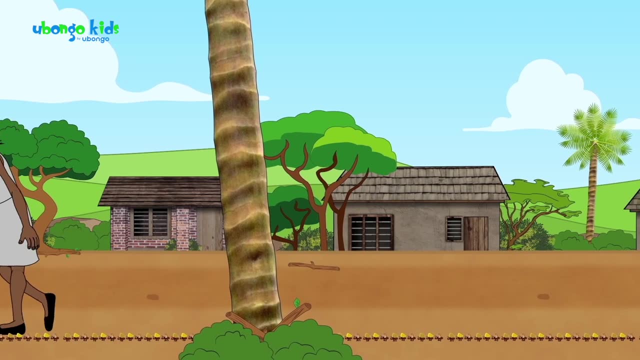 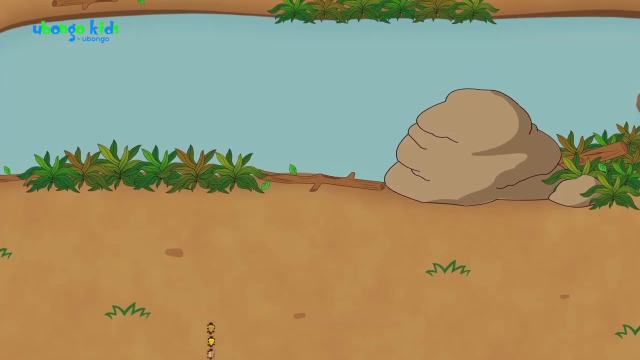 and a drawing of a house. What if this code is giving them directions to get home? I'm going to follow them and see: One, two, three, four, five, six, nineteen, twenty. I ran twenty steps And now they're turning right then going straight towards the pond. 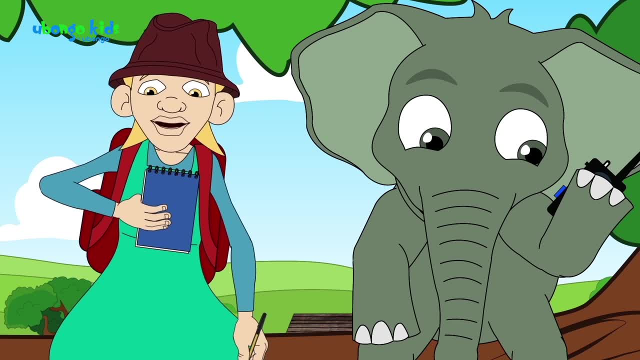 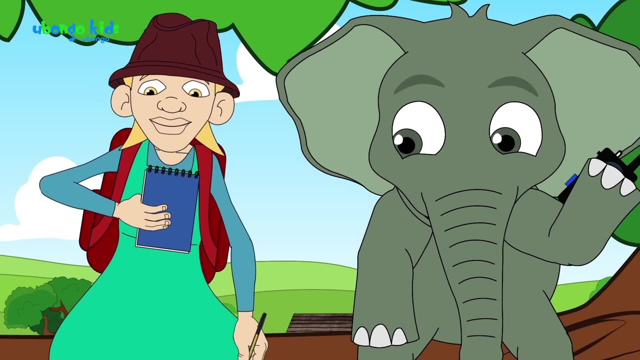 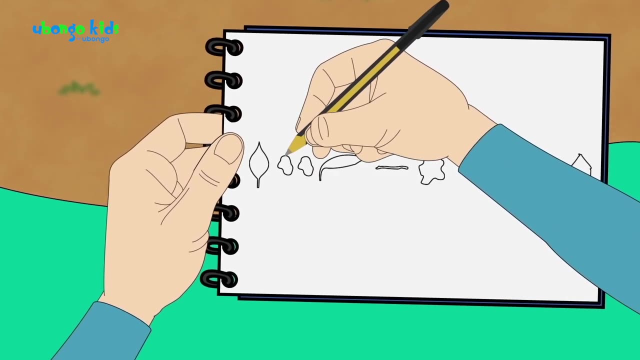 The code shows two rocks, then a right turn, then a straight line right up to a pond. Two rocks, two rocks. When I run, each step is about a meter. What if one rock means ten meters and two rocks would be twenty meters? 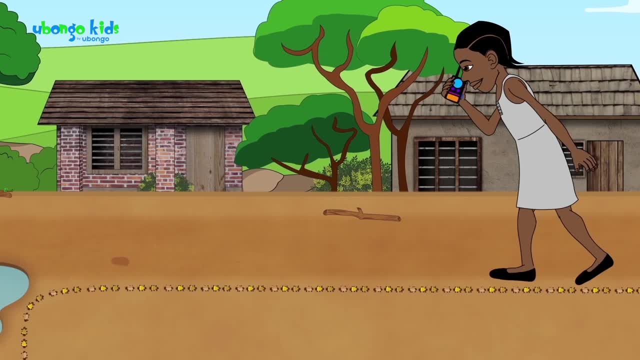 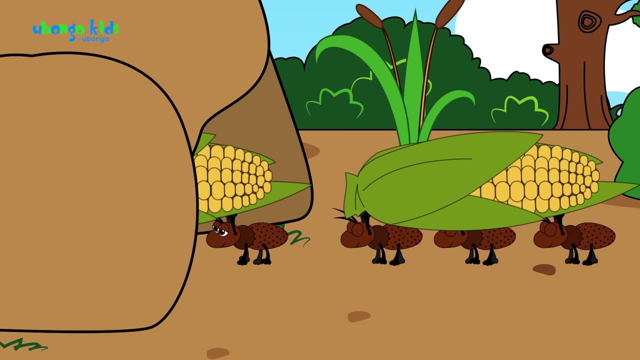 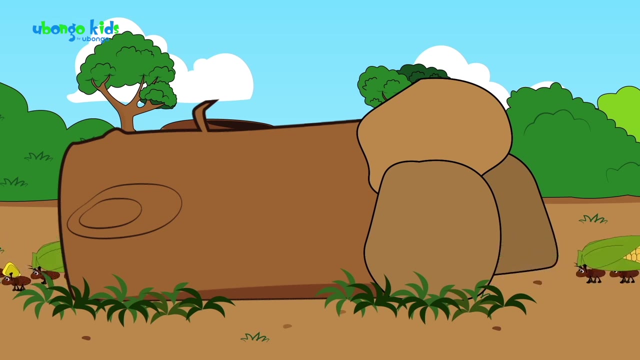 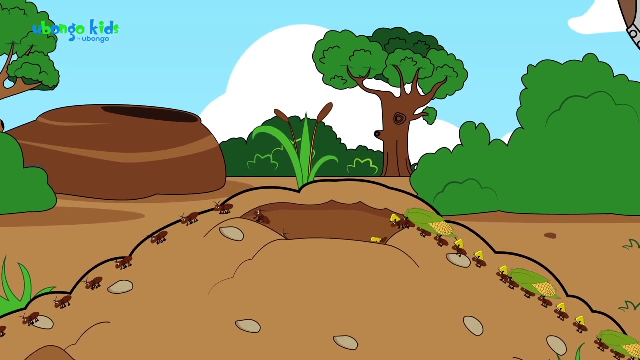 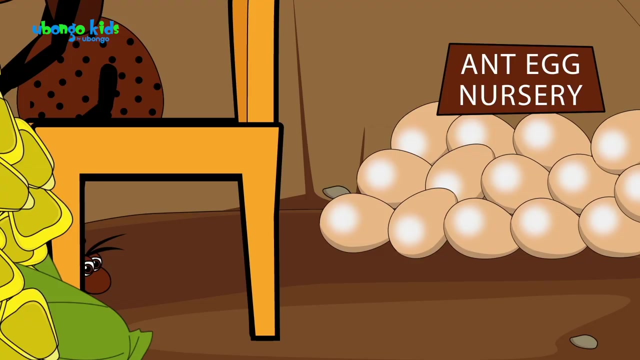 And a straight line to the pond. So what if that means go straight until you reach the pond? The only way to know is to check. I think we're on our way to cracking the code. I found their queen And whoa, she can eat. 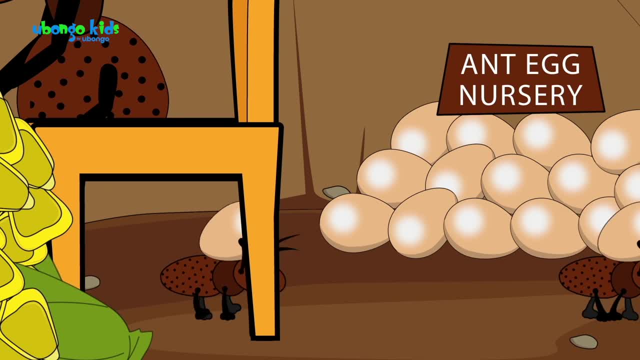 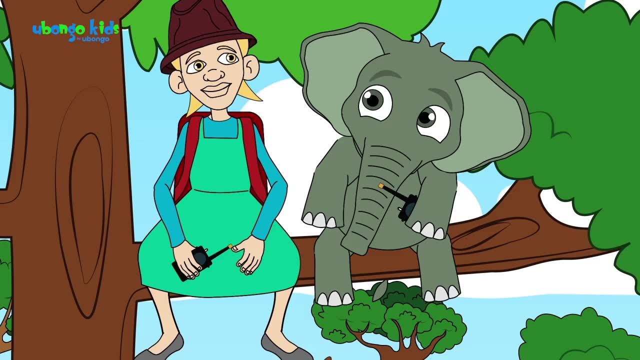 Oh, so that's why they're taking so much food. The queen is eating it so she can lay her eggs. Five, four, three, two, one. Okay, now we've answered two questions. One: why do the ants take so much food? 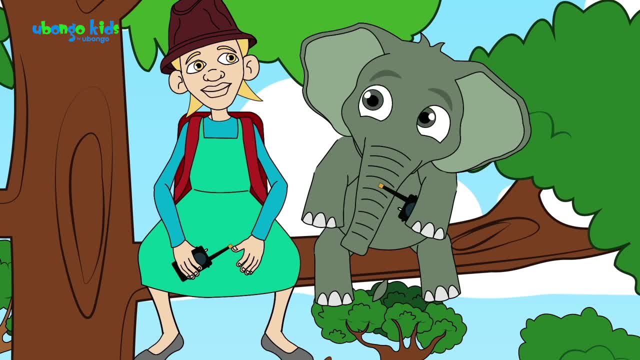 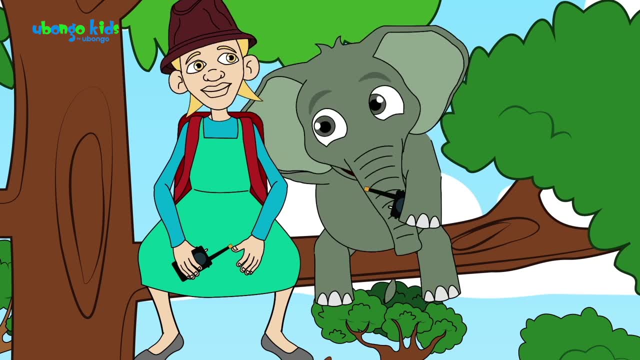 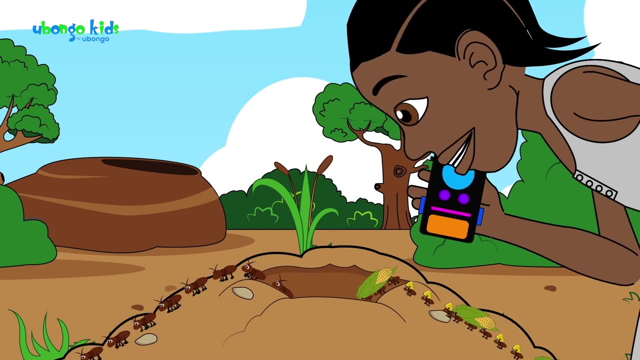 Because their queen needs it to lay lots and lots of eggs. Two: how do the ants communicate? By using leaves and symbols as a sort of code To tell each other where to go and what to do there. Well done, guys, But to solve the conflict we now need to answer the third question. 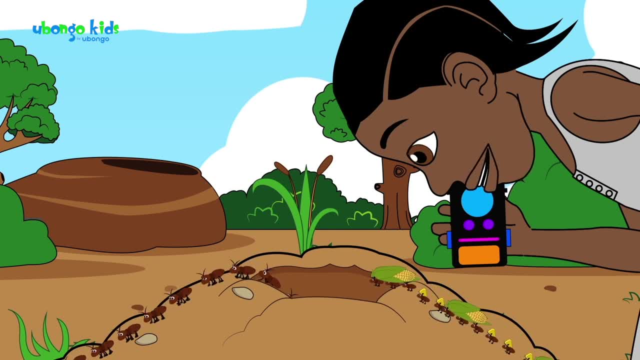 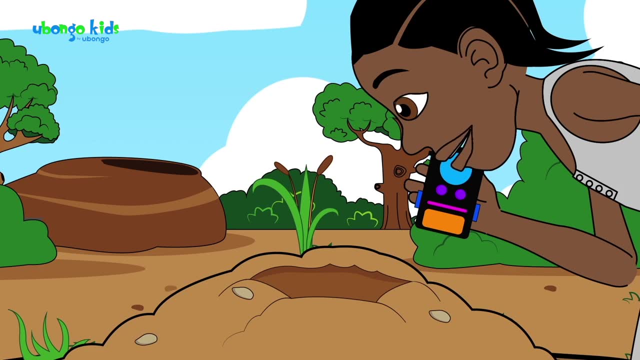 Where can we tell the ants to go instead, so they don't steal food from people in Kokotoa? Question number three: Well, I think I figured out what the squiggly leaves mean: Ant dance- We're starting to understand them. 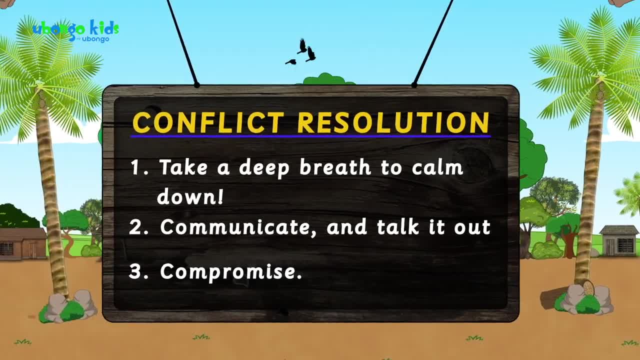 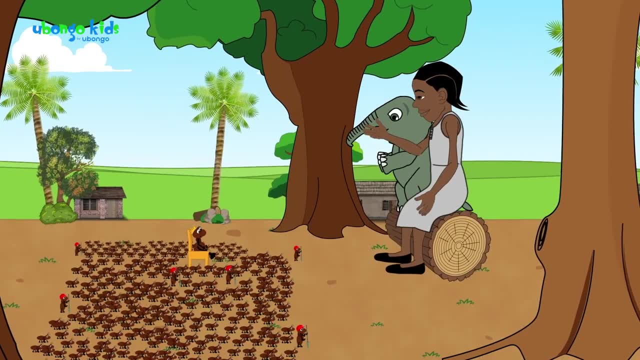 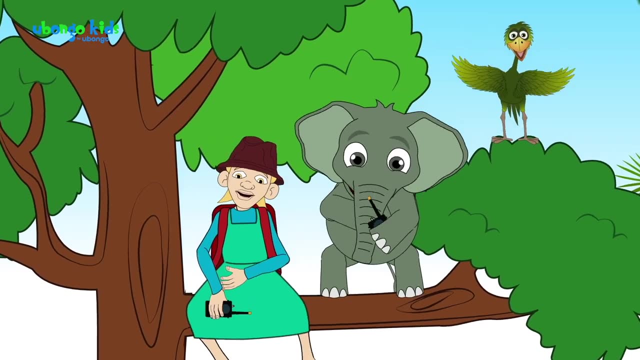 Now we can solve the conflict. When we get in a fight, we each think we are right. We have to sort it out and find a way To listen to each other, understand one another. We can work together to make it okay. 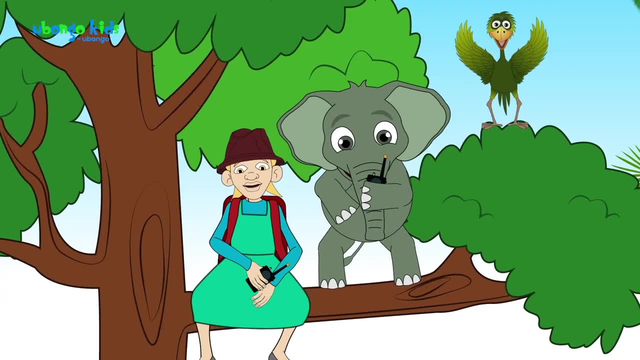 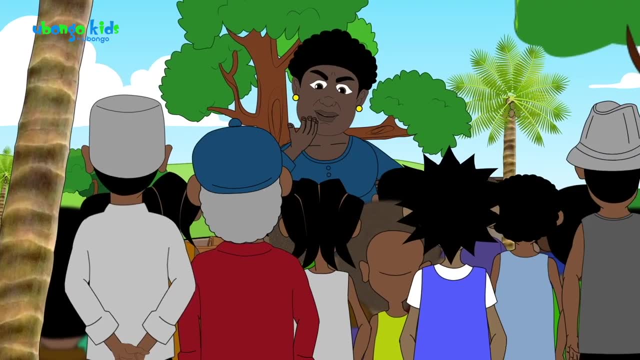 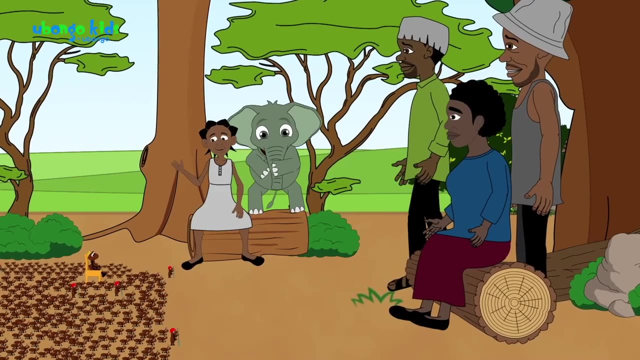 I need to tell you how I feel. You need to tell me how you feel, Then we'll take a walk in one another's shoes. We gotta compromise instead of taking sides, Then neither of us has to lose. This is a conflict resolution song. 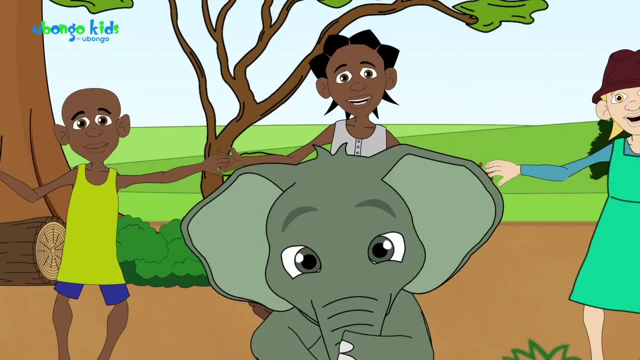 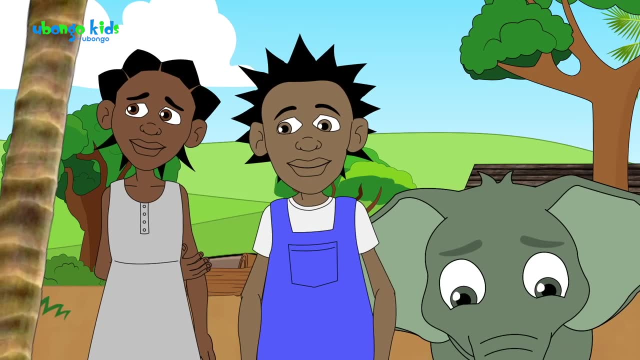 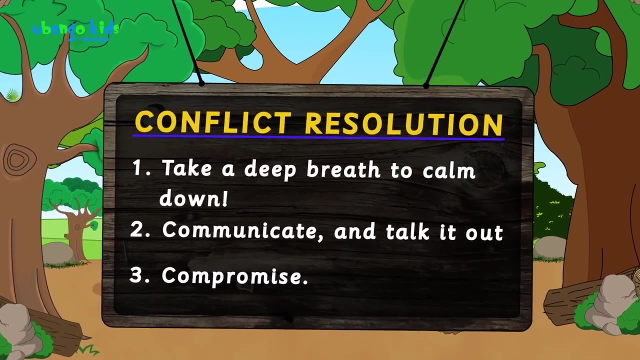 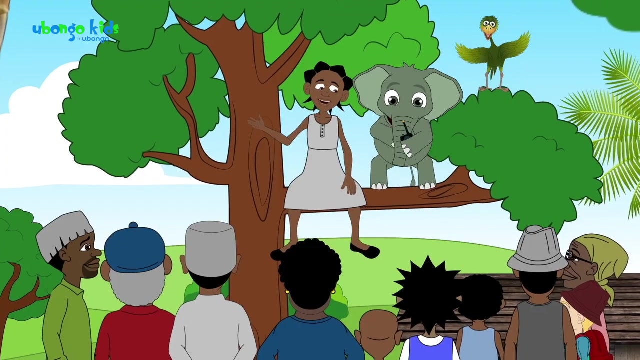 We will use it to get along and live together in harmony. When you're in a conflict, stop first and think, Then follow these steps to solve it peacefully. Step one: take a deep breath to calm down. Step two: communicate and talk it out. 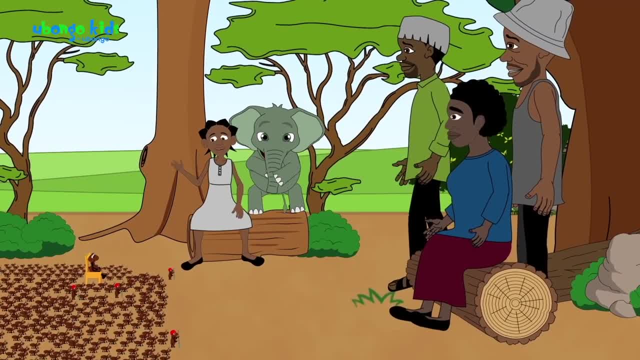 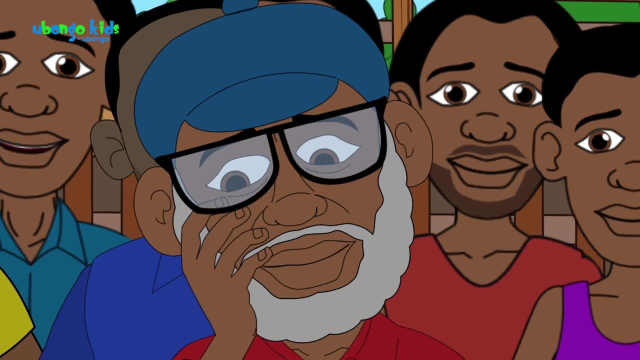 Step three: compromise. You each have to give to get a solution. you can both live with. Step one: cool down, Take a deep breath. You can't solve a problem when you're so upset. Step two: talk and listen to the opposition. 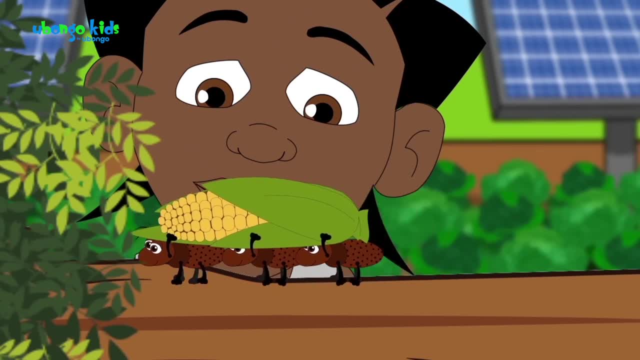 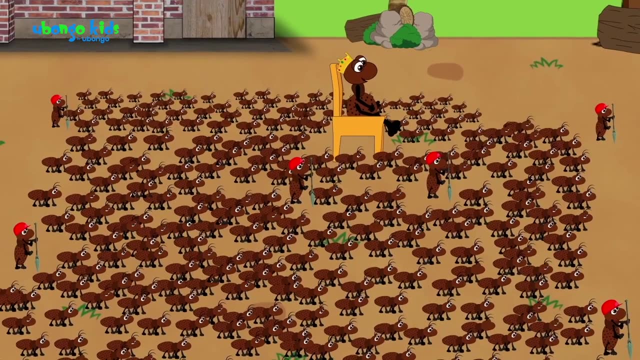 What do they want? What do you want? Take a walk in each other's shoes. Understand what the other has to lose. Step three: compromise. It's give and take. We each give a little for the other's sake And at the end of the day we can walk away. 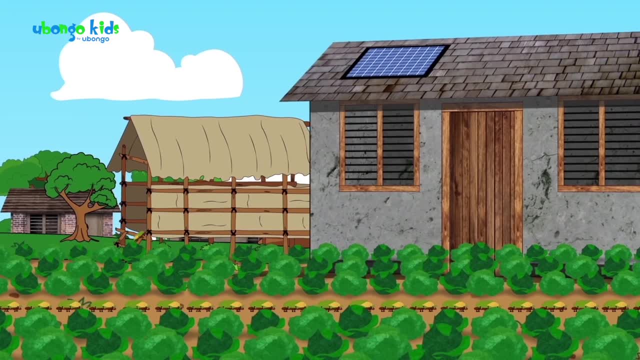 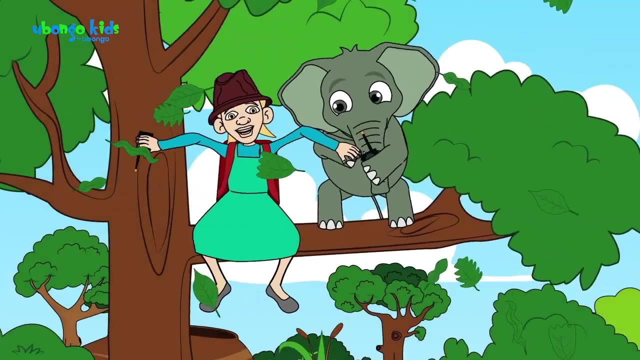 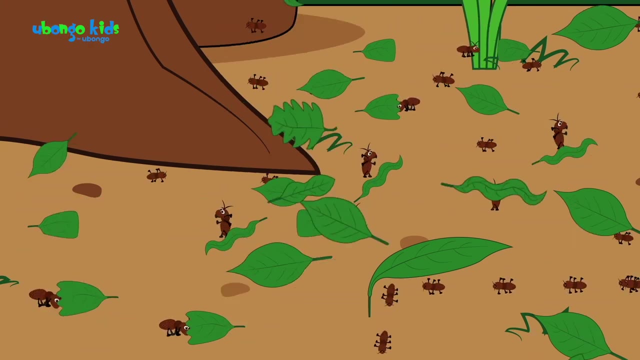 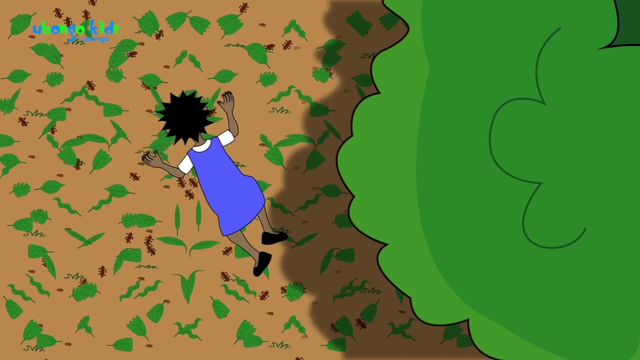 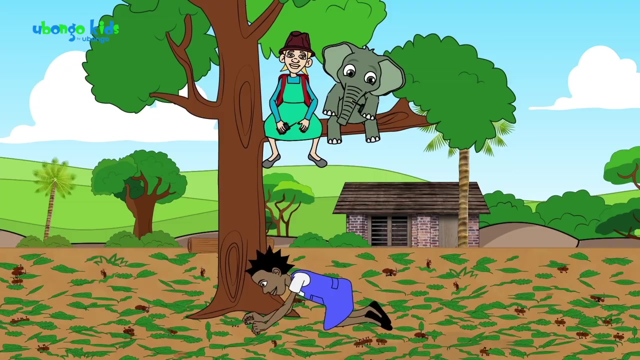 Knowing that we solved the problem peacefully So we can live in harmony. No, The leaves. Red alert, Repeat Red alert. The ants have gone wild. We need help. Tiny Timbo, I'm on it. Red alert, Red alert. 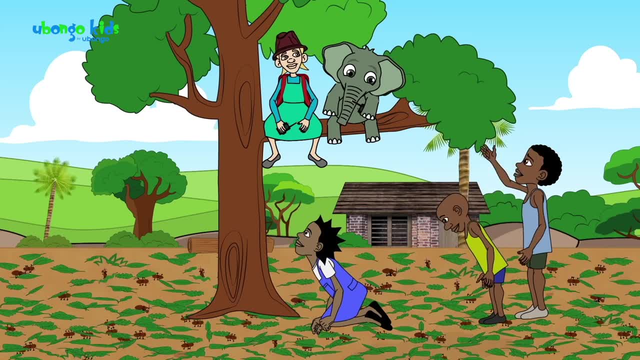 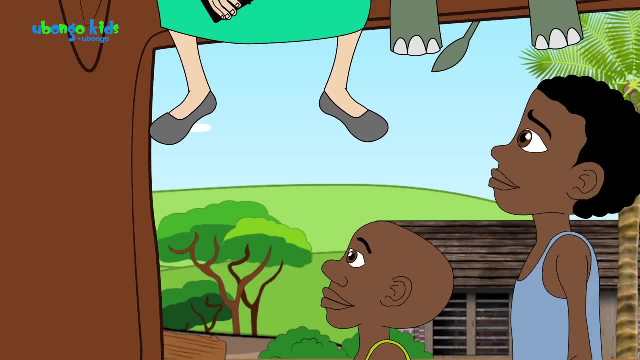 The ants are going wild. Okay, tell us what to do to help Koba Baraka Kiruchu. You need to use the leaf code to bring all the ants back to one place And keep them away from people's food and crops. 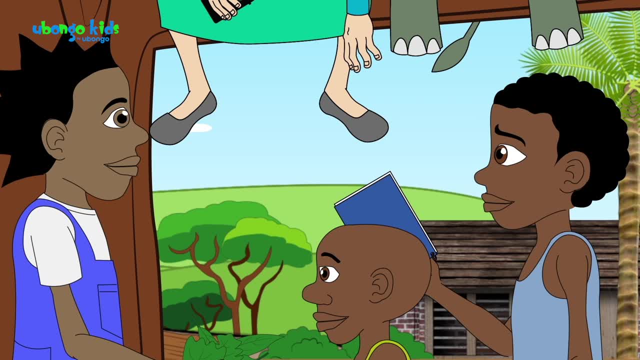 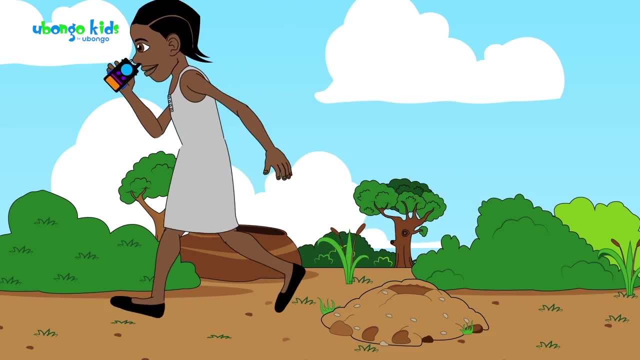 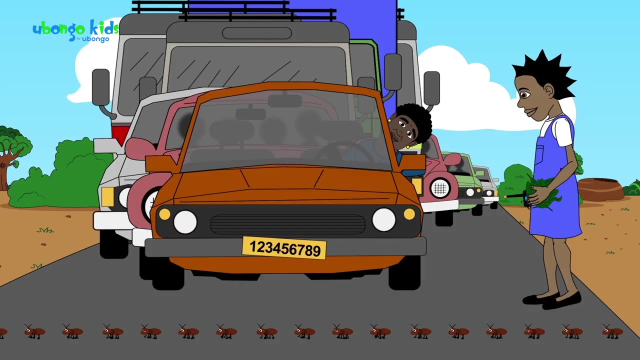 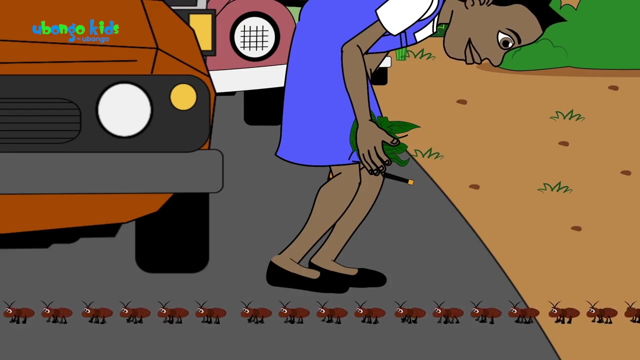 Copy that, Kibana, you need to figure out what else the ants will eat So that we can send them to a new location. Copy that. It's those ants again, Always causing trouble. Tomorrow we fight. Try a long, skinny, pointy leaf. 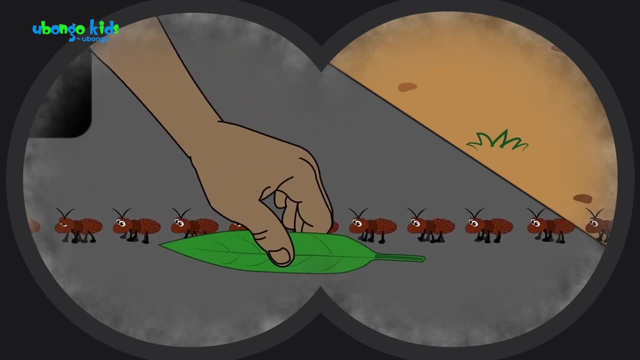 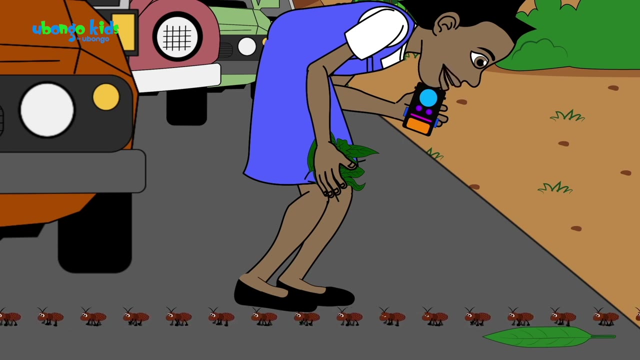 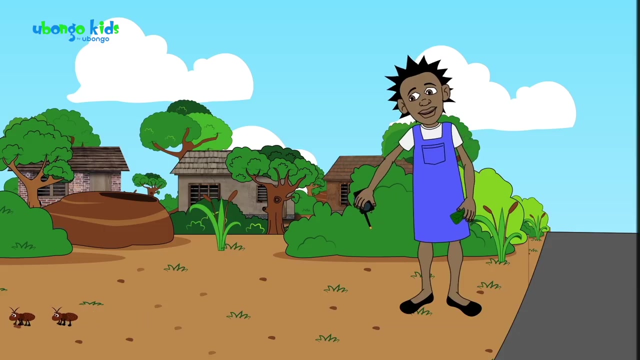 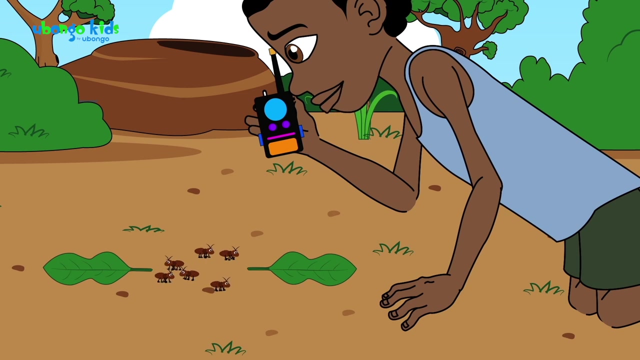 I think it tells them to go faster. Uh-huh Confirmed. The long, skinny, pointy leaves mean move fast. Oh yeah, Oh, Stop, Stop, Stop. The leaf shape like number eight means reverse: The ants turn around in the opposite direction. 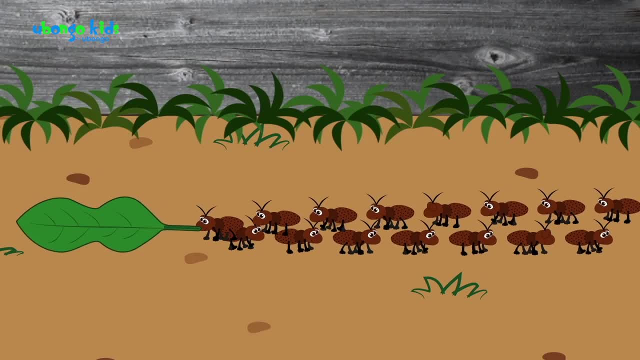 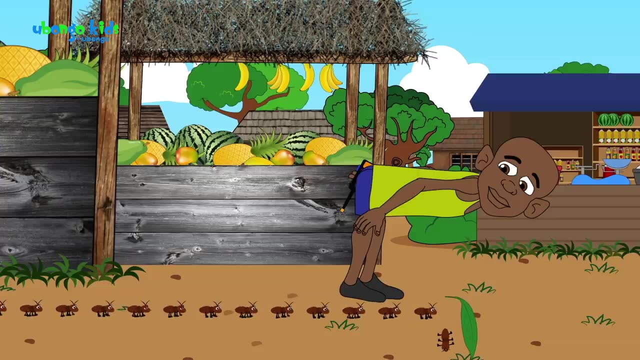 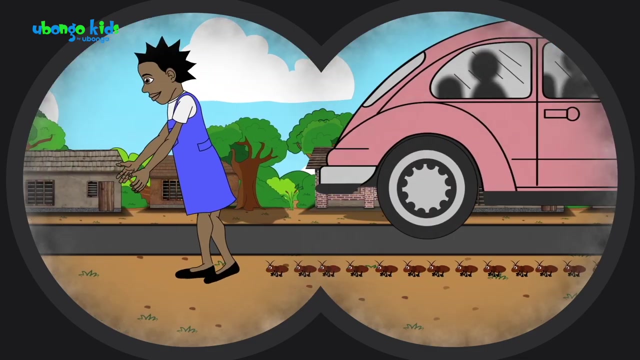 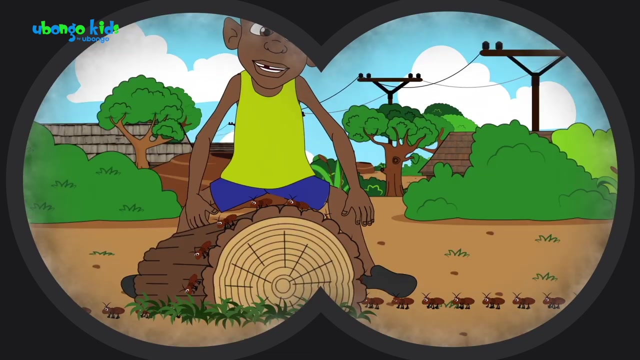 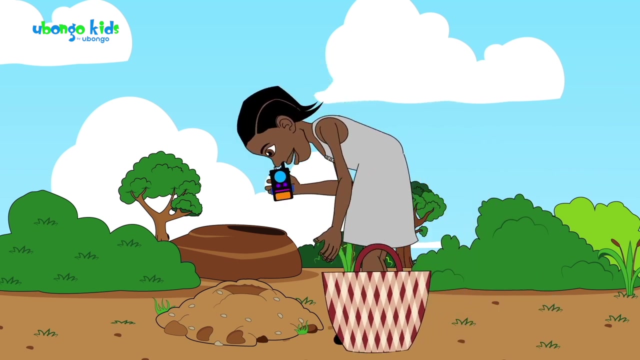 Just in time. Good job, guys. You really got the code down. Amani to Kibana- what's your status? I'm testing different items to see what else the queen might like to eat instead of Kokotoa's food supply. 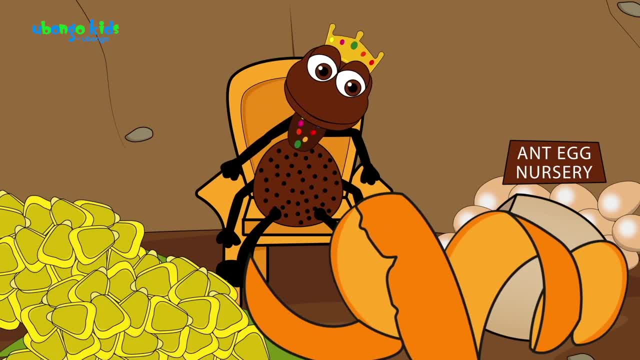 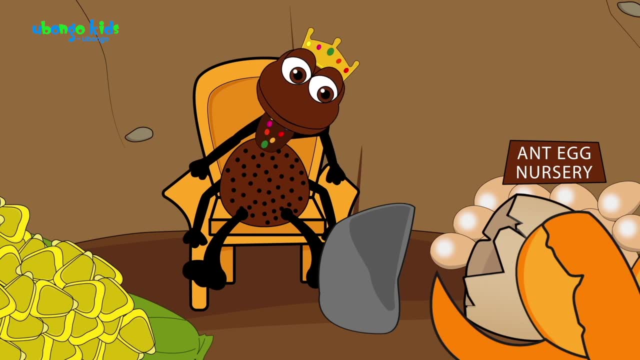 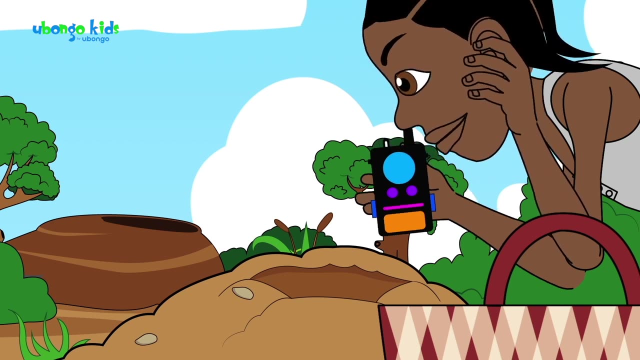 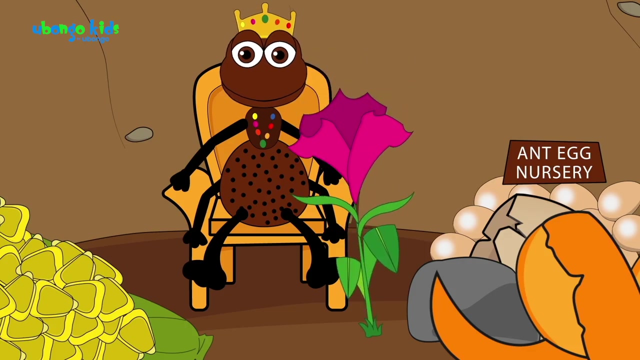 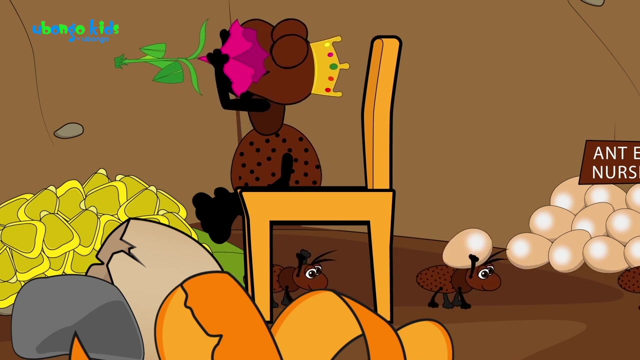 Hmm, Not eggshells And not fruit peels either. She doesn't like pebbles. No one eats pebbles. Kibana Flowers. She likes the flower nectar. We can use the code to redirect the ants to the flower. 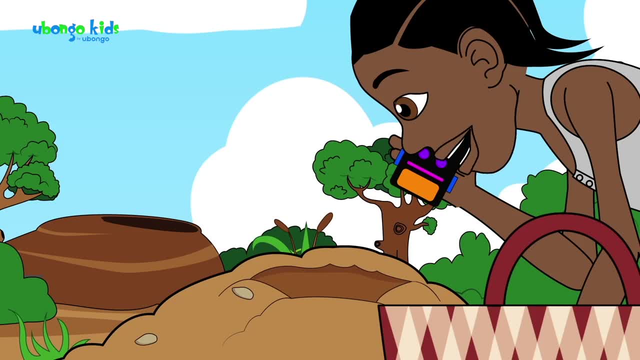 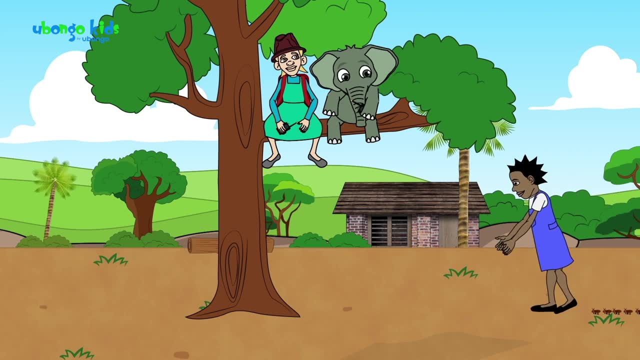 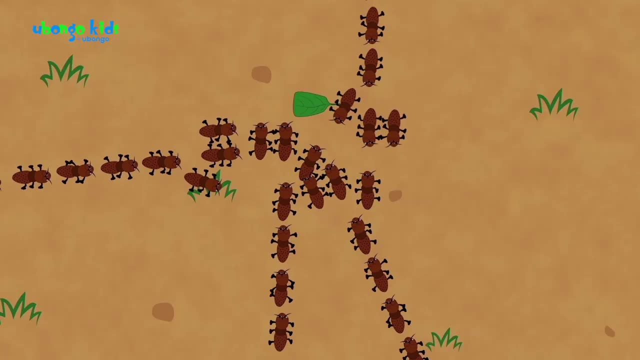 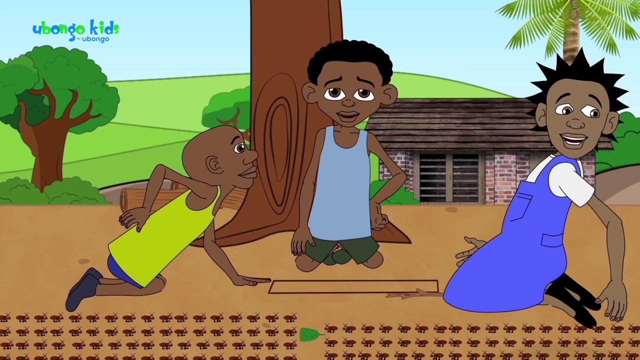 To redirect the ants to the meadow to collect flowers. Question number three answered. Now let's get you guys back to the tree. Let's use the code to give them a series of instructions which will lead them to the meadow. Amani, can you see the meadow from up there? 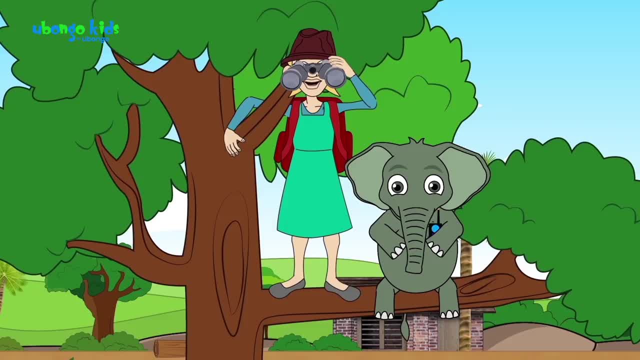 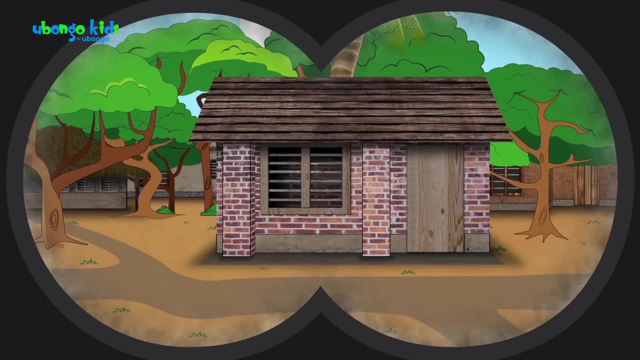 Tell us where to send them. I see it. We need to tell them to walk all the way towards Kibana's house, Then turn left. I think you need to add a symbol to what you want them to go straight to. I guess you need to add in a symbol. 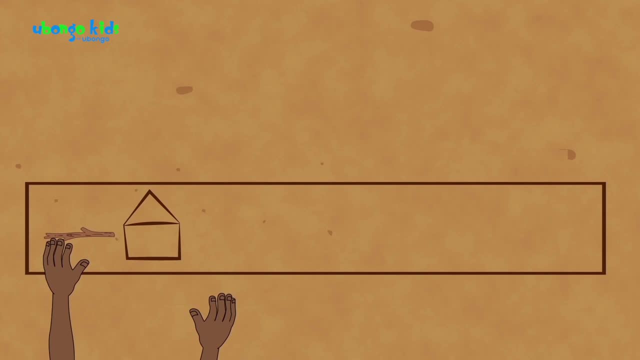 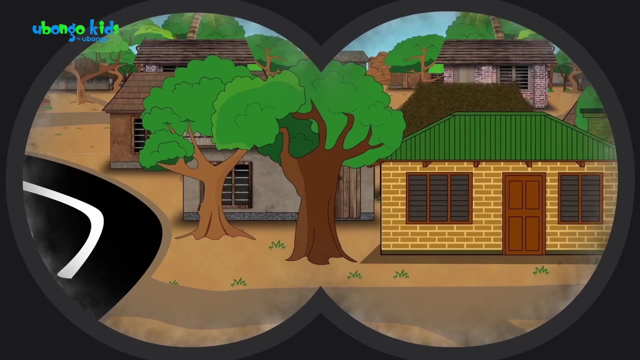 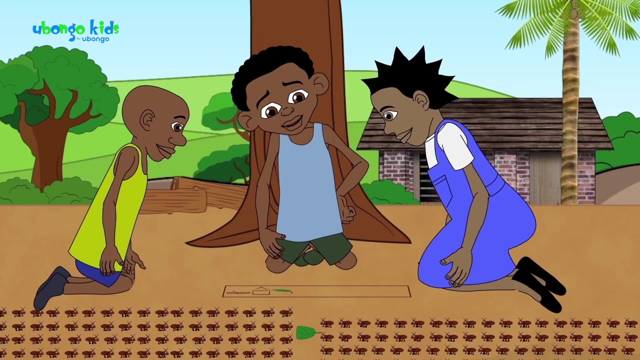 for what you want them to go straight to? Ah, Nice, drawing Baraka When we need them to turn left, Then from there the ants are going to have to cross the big road, Or we could have them tunnel under it by using a dig leaf. 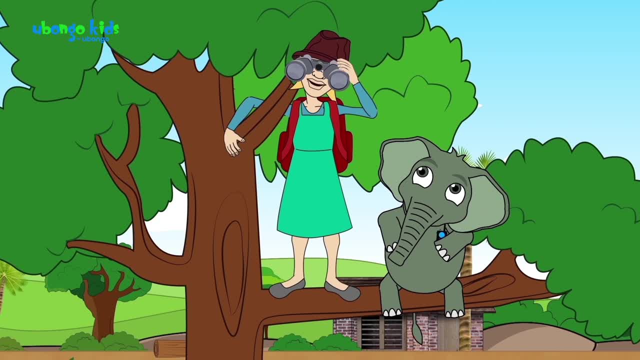 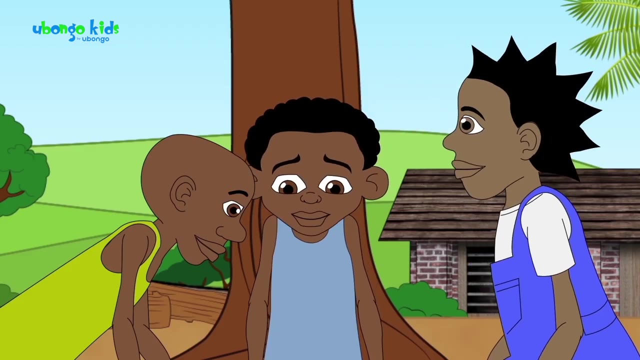 This leaf means to dig down, And from there they need to go forward Um 40 meters. Remember, guys, a rock represents one meter, So four rocks means 40 meters. And what next Looks like they just need to walk straight. 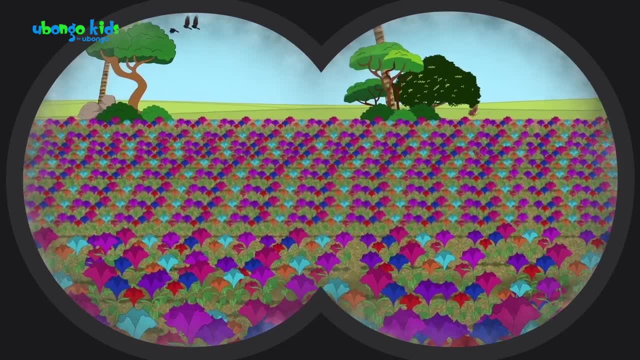 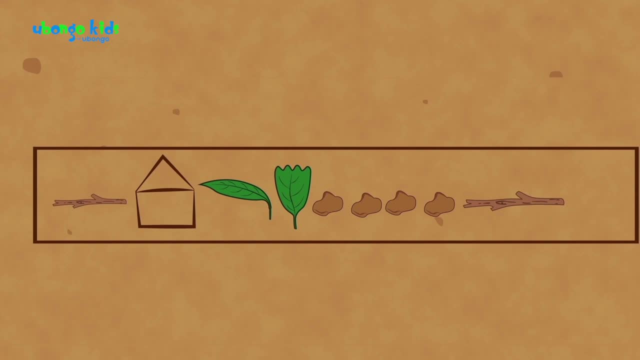 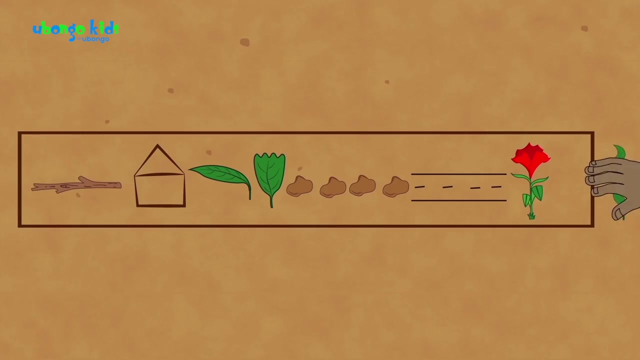 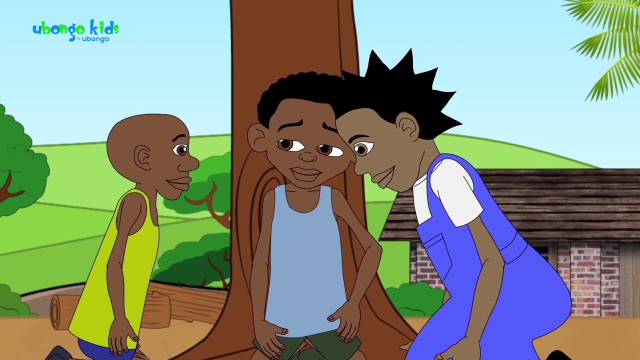 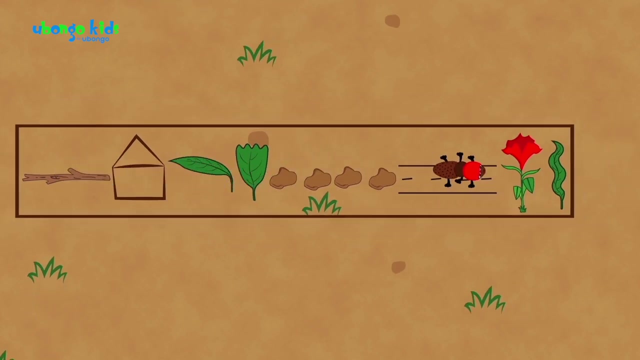 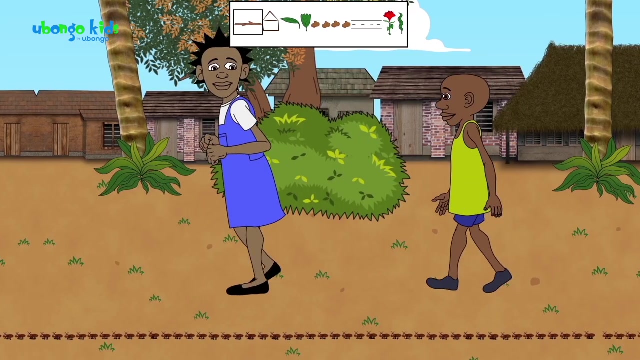 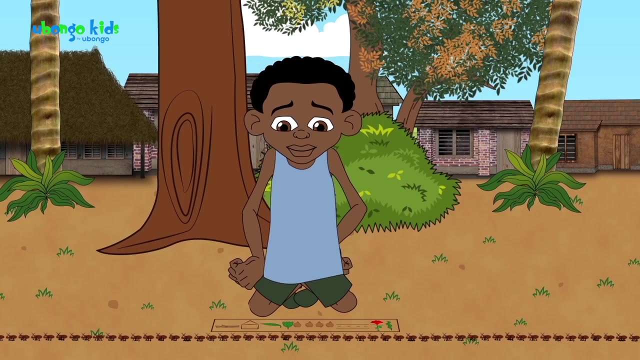 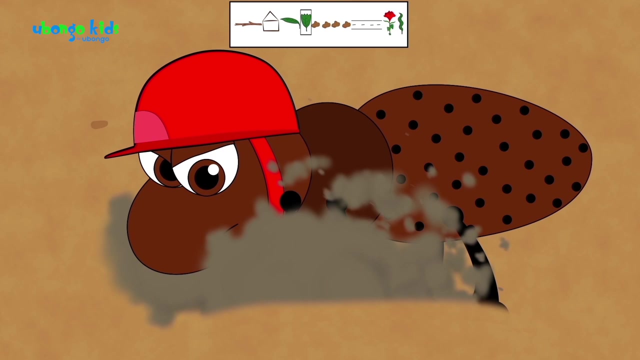 until they reach the meadow. This means straight to the flowers, And let's make sure they do a little dance to celebrate their happiness when they arrive. I think we're ready. No, Why is she digging? They're not supposed to dig. 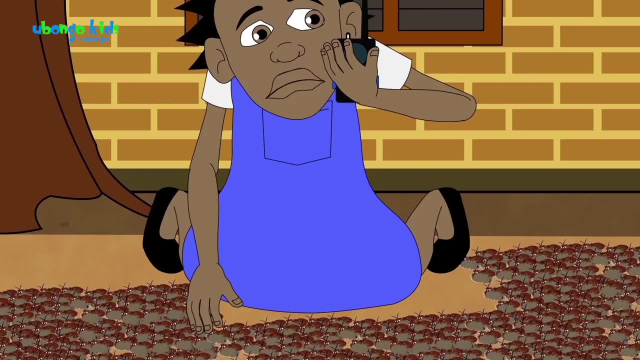 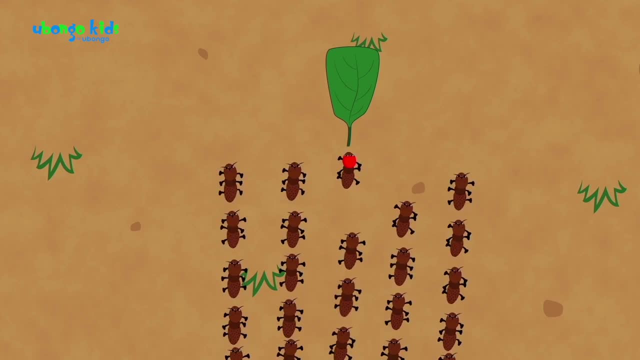 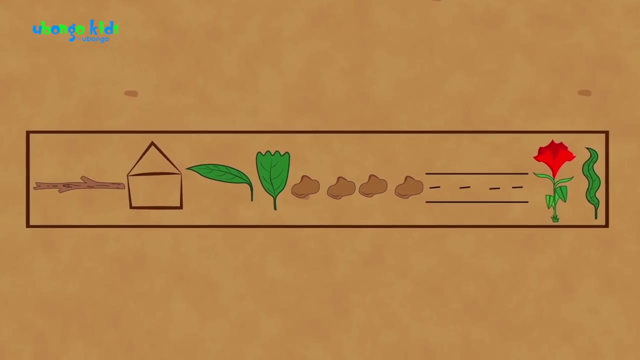 until they get to the road. Red alert. Red alert: Use the code Kiduchu, You can figure it out. Aw man, we messed up. We put the dig leaf right after the turn left leaf. We didn't give them any instructions. 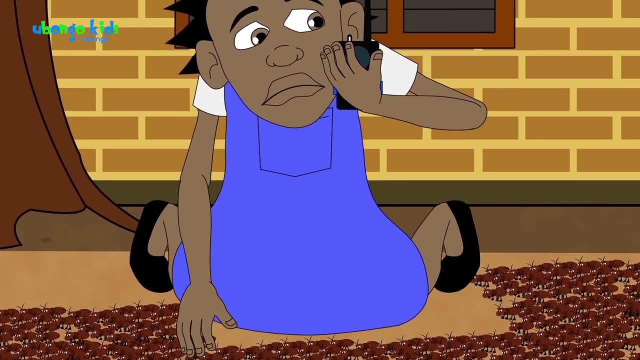 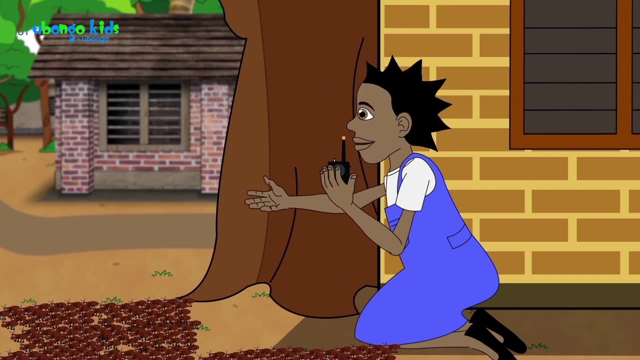 to walk to the road first. Kiduchu, you're gonna have to write a new code there. Hmm, the road. They need to go to the road before they dig. I need a stick Straight to the road. dig, go 10 meters. 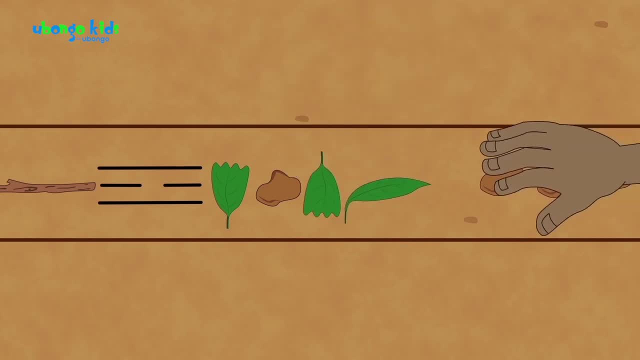 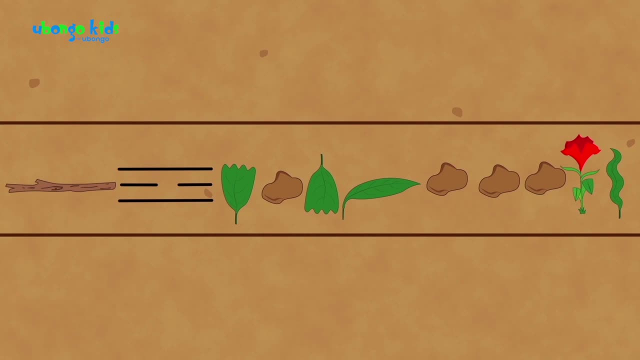 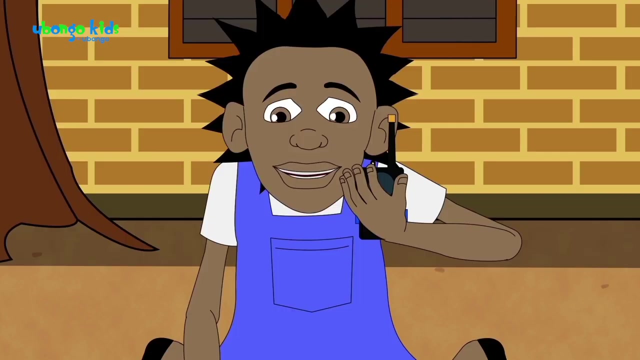 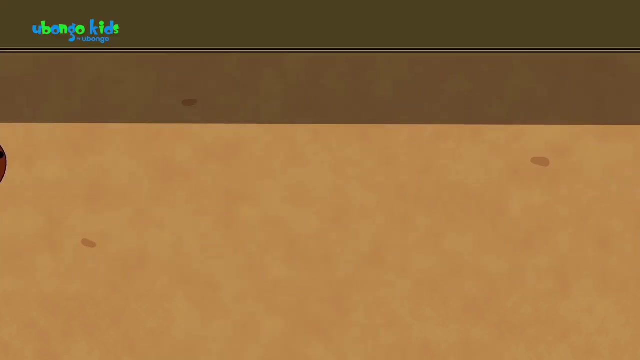 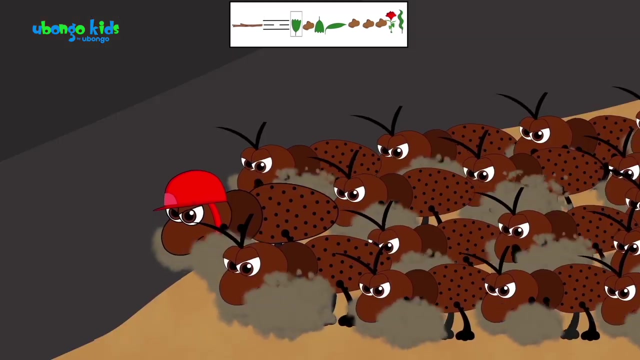 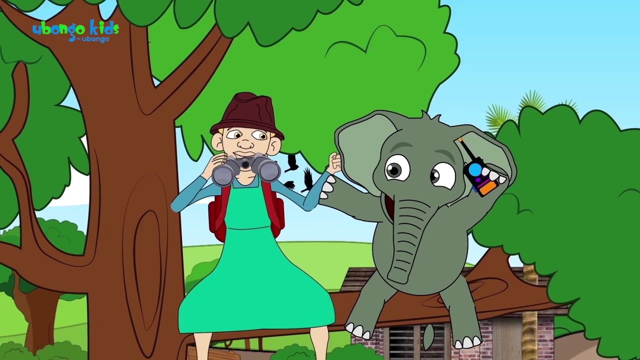 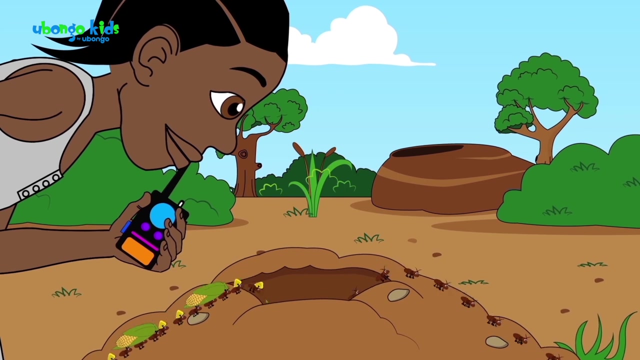 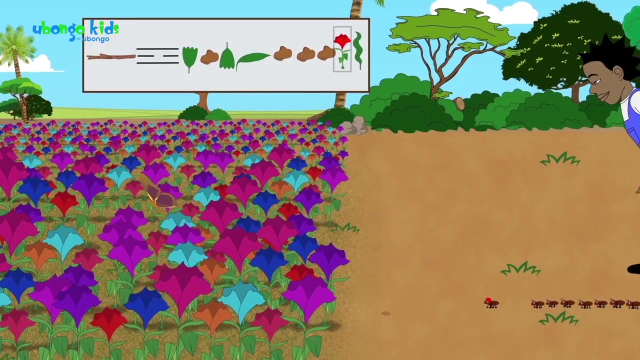 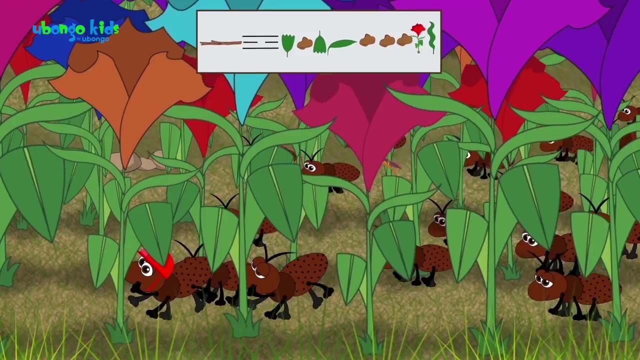 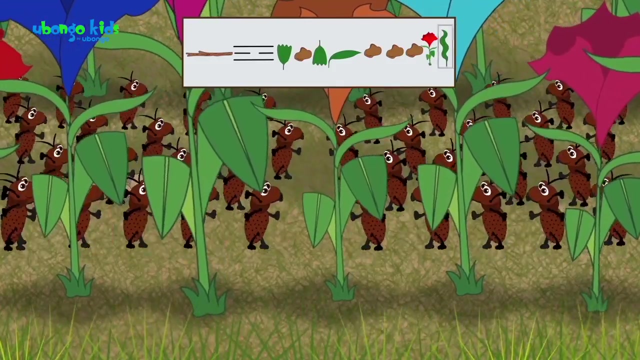 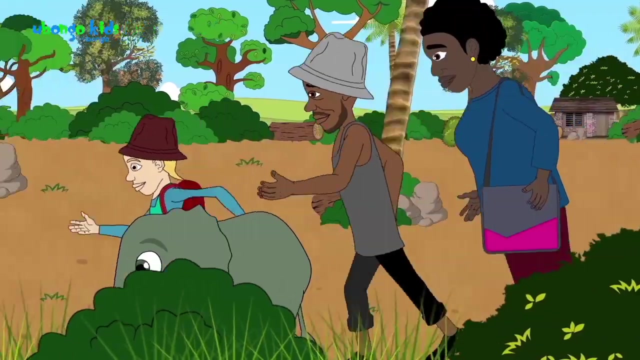 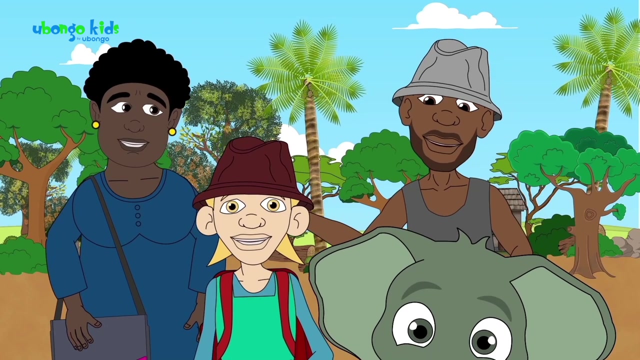 Come back up, turn right 30 meters to the flowers And don't forget to dance. Code fixed Time to try again. Yay, It worked, guys. Come on, It worked. Look. Ah, well done kids. 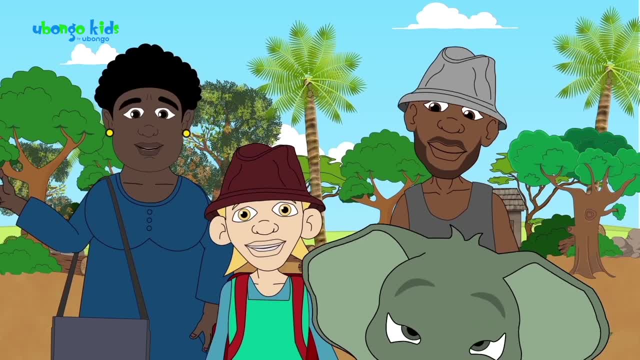 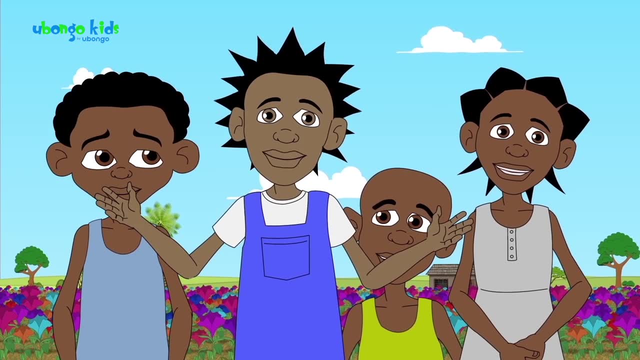 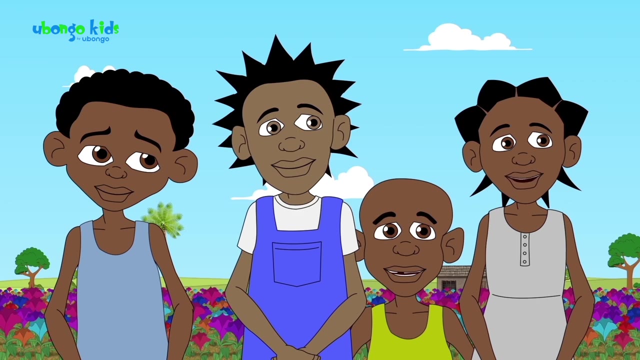 Good job, Kibena, But how did you do it? Well, we had to watch and learn So we could understand the ant side of the story. They were taking extra food back to their queen. She needs lots of food because she lays all the eggs. 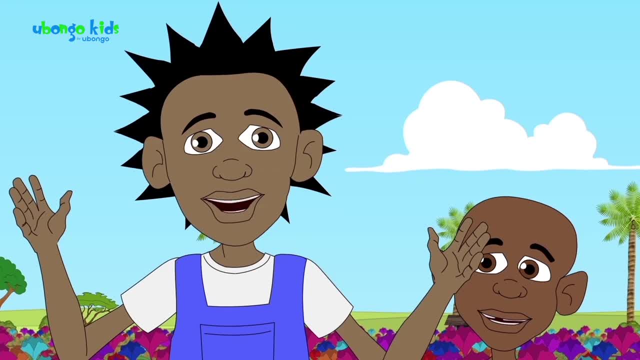 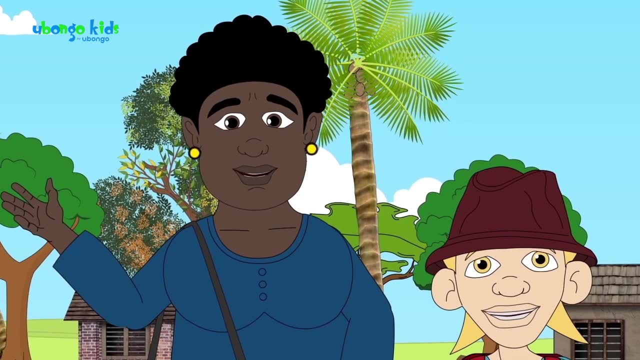 And then we had to talk to them to get them to come here instead. But they don't speak in English, They use a code Aha, Like a computer code. What's that? It's how we computer programmers communicate with a computer or a phone. 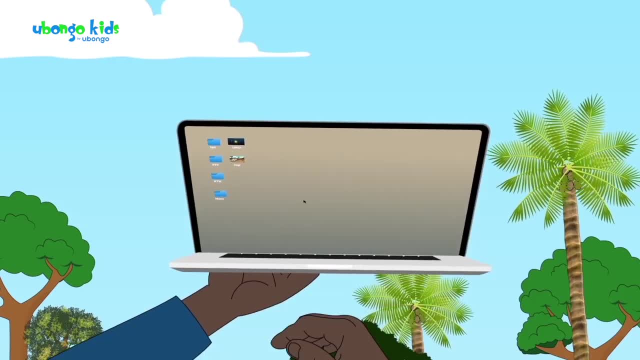 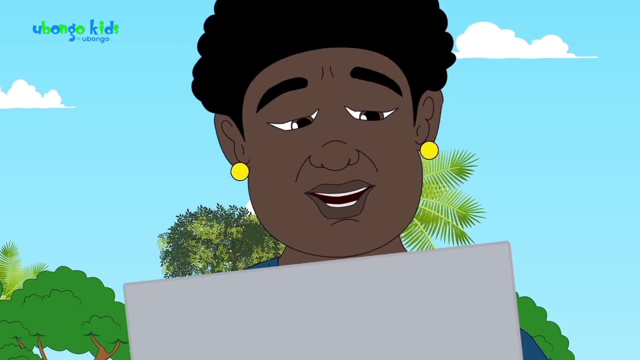 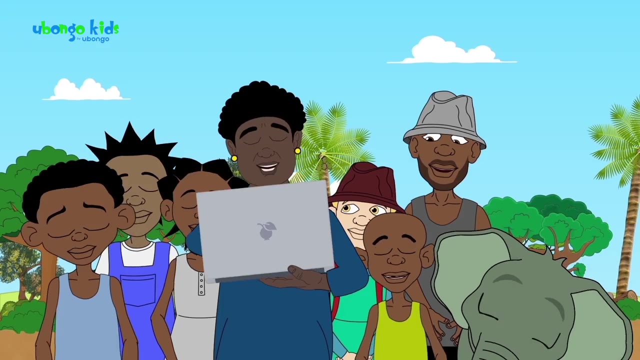 It's a set of instructions that tells it what to do in different situations. You know I'm a busy woman, So I use code to create programs that tell my computer and phone what to do. Hmm, Let me give you an example. 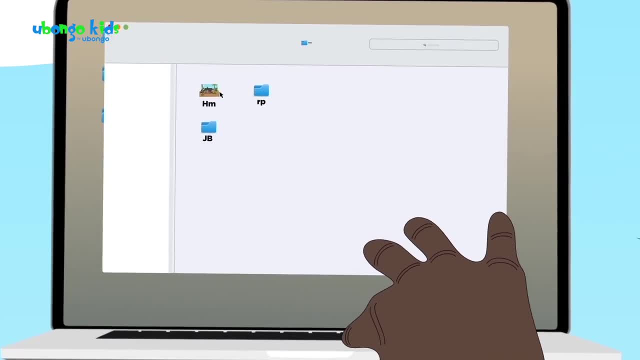 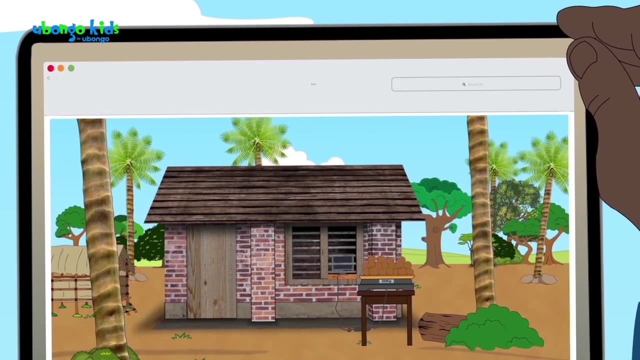 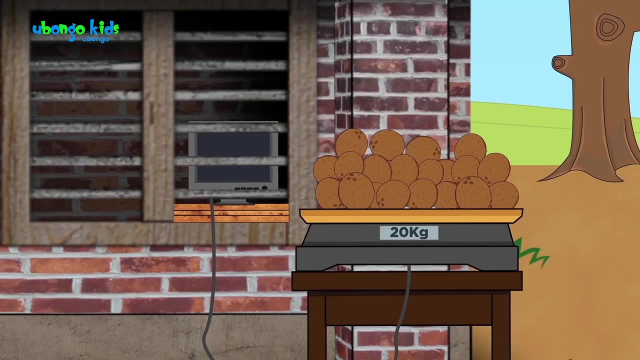 You know I sell coconuts right kids, But I also teach computer classes. I can't be in two places at once, So my computer and phone control my coconut business While I'm away. Pretty neat right. Each coconut weighs about one kilo. 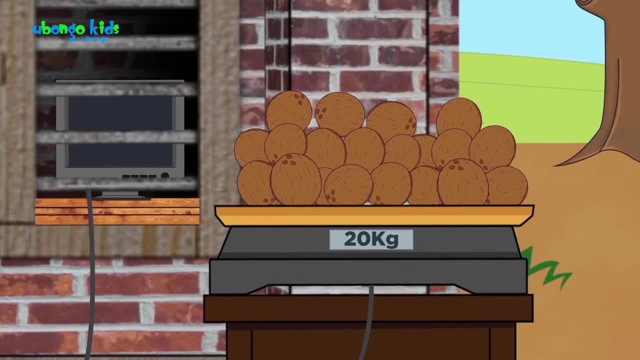 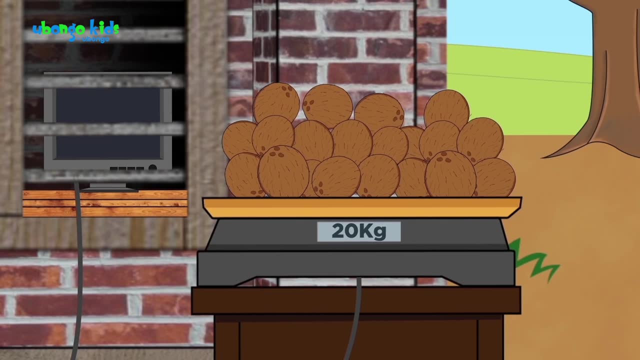 And I leave them sitting on a scale that is hooked up to my computer. So I start the day with 20 coconuts on the scale, weighing 20 kilos, And I leave them there. I have coded a program that tells my computer what to do to manage and sell the coconuts while I'm gone. 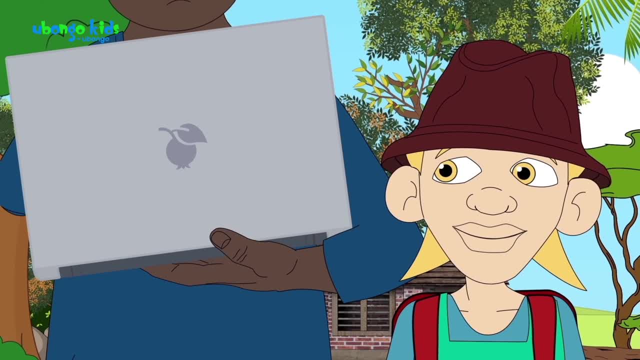 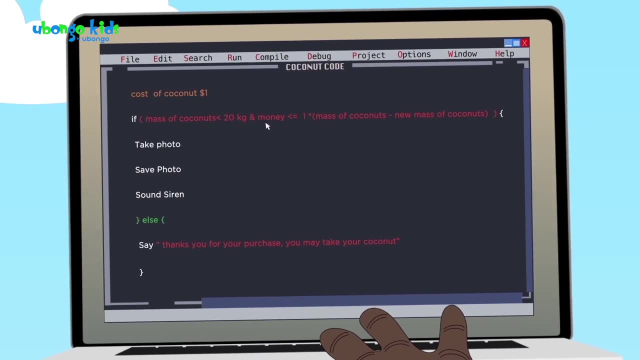 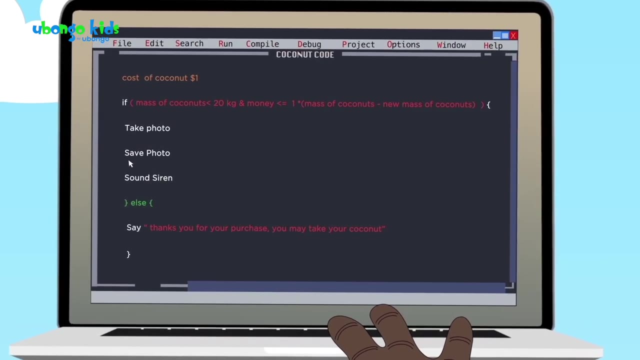 But how Don't people just steal the coconuts? Huh, They'd better not. My computer code says: if the weight on the scale decreases, then take a picture and make a loud, scary noise. Then I have another command that tells my computer to save the photo. 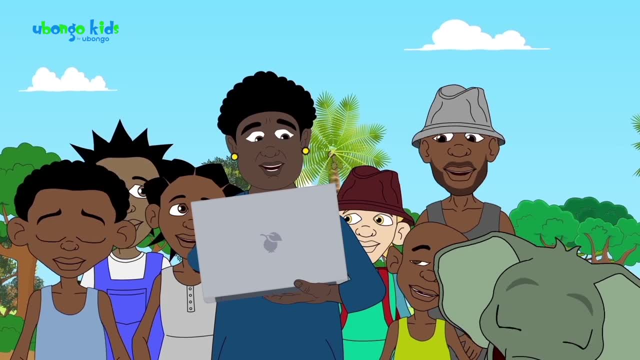 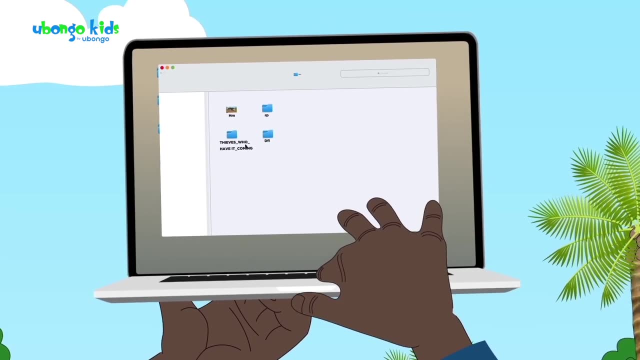 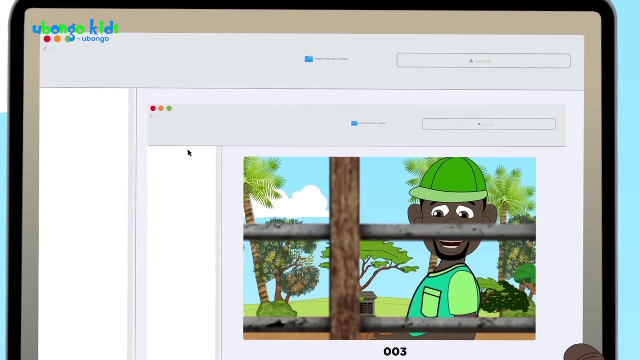 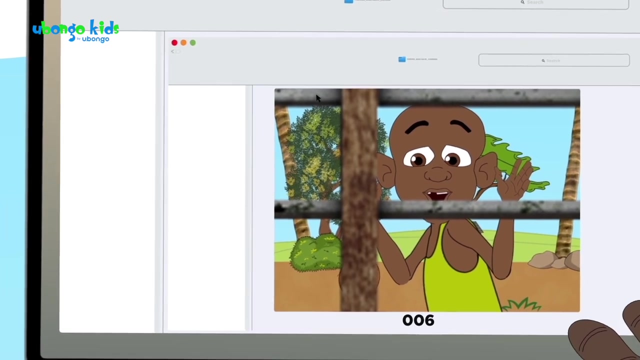 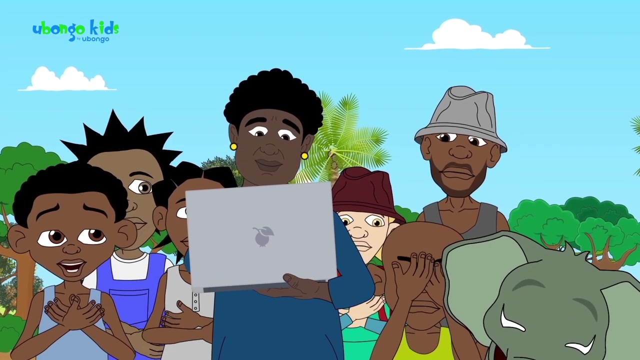 And then whoever is in the picture better watch out. One, two, three, let's go do it, And here's your money. Baraka, Uh huh. He's learned his lesson and already paid it off in full by climbing trees and collecting coconuts. 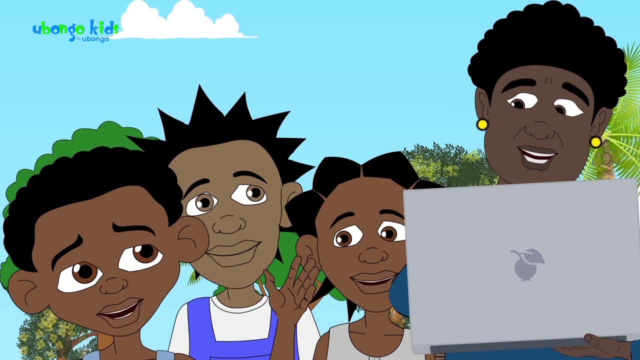 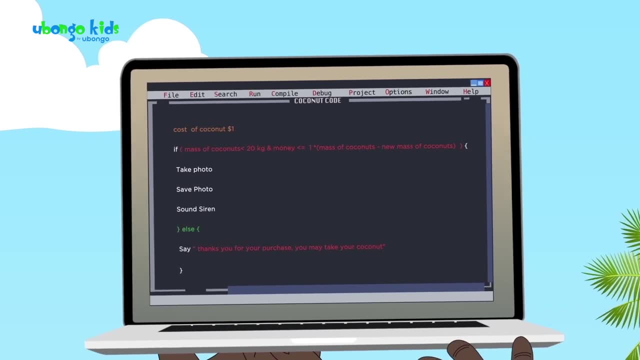 and collecting coconuts. But how does your computer sell the coconuts while you're at school teaching? That's another part of the code within the program. It says: when my phone receives a payment of 1,000 shillings. 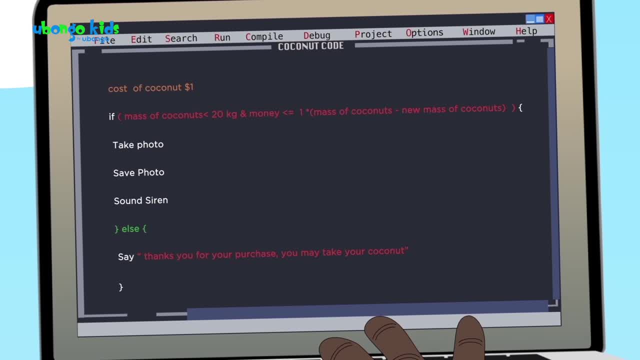 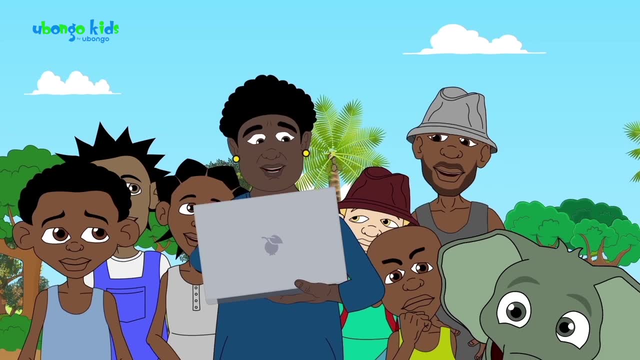 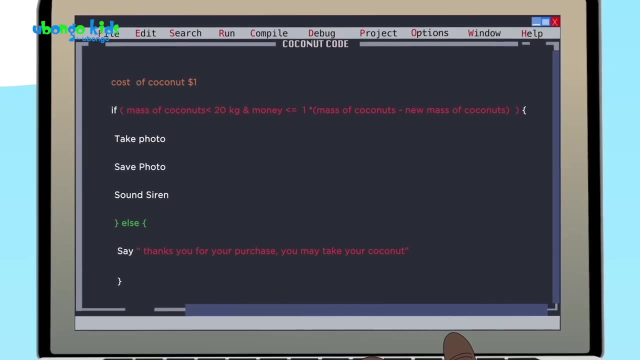 then play this audio. Thank you for your purchase. You may take your coconuts And if the weight reduces by about 1 kilo, then it stops the program for the photo and siren. If it reduces by any more, then 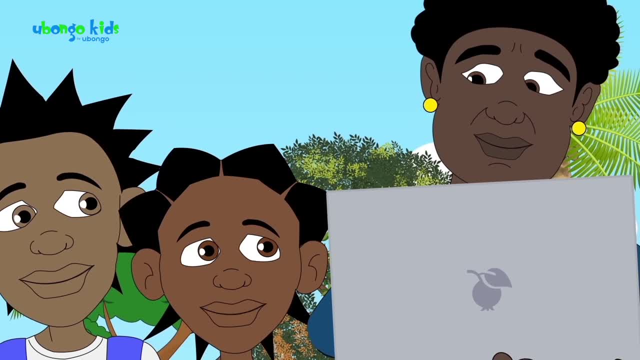 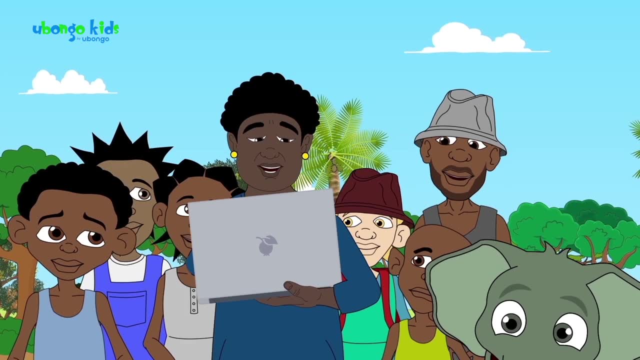 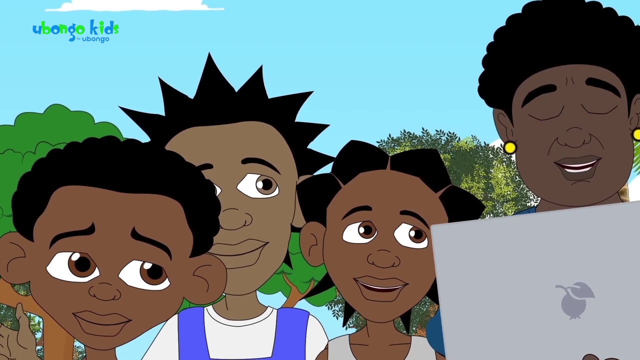 So that's computer code? Yes, It's just the instructions I've given the computer, which it then carries out, And I'm adding more code every day. We used a code kind of like that to tell the ants where to go, And we hope now. 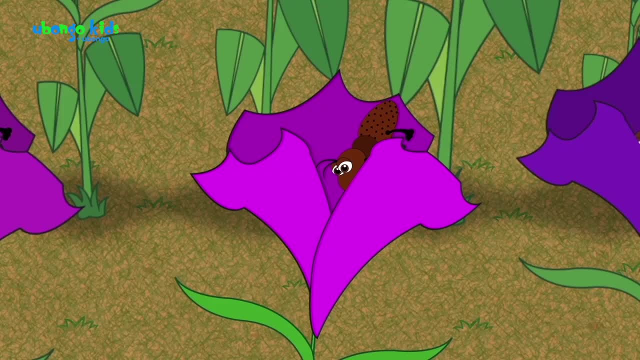 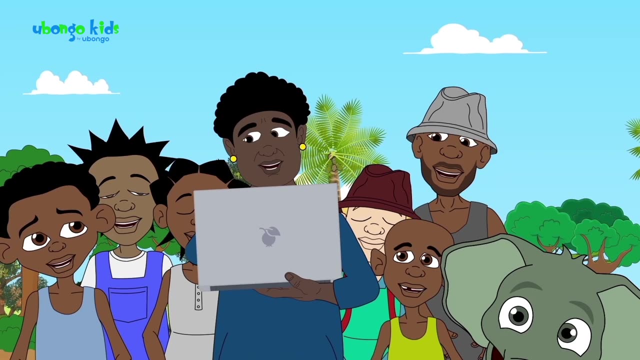 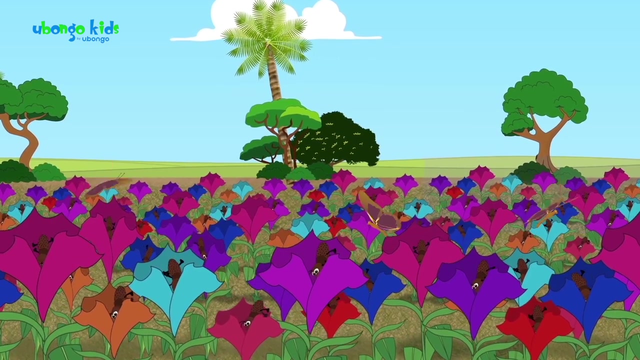 they're getting their food from here instead of the village. You'll be willing to keep the peace. Yes, This is a good compromise between the humans and the ants. We will give them this beautiful meadow in our village so they can have all the flower nectar they want. 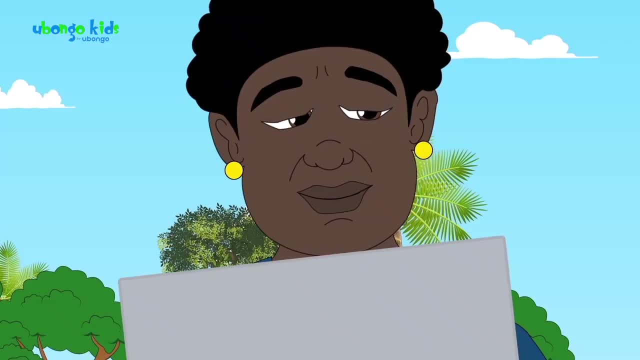 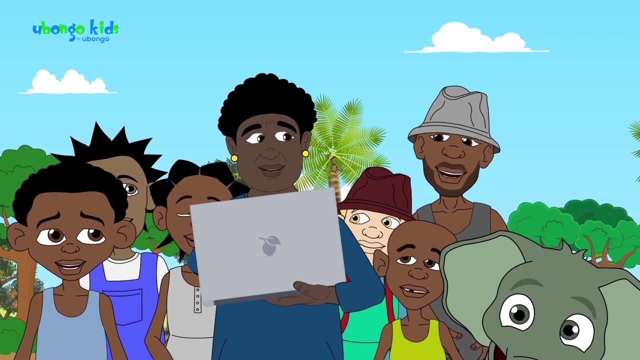 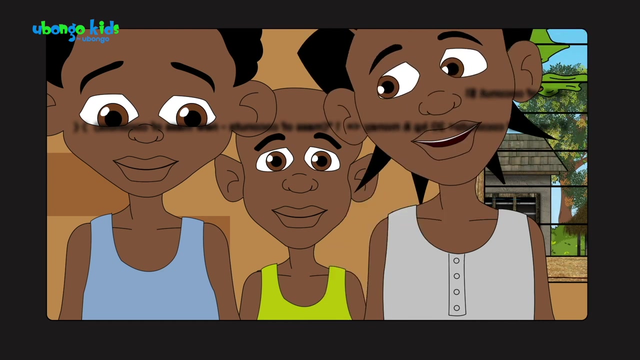 And in return, they'll stop stealing our food. With this compromise, I'll keep the peace, But I want one thing from you: You kids need to keep coding. Where do we start? What do we do? This coding thing is completely new. 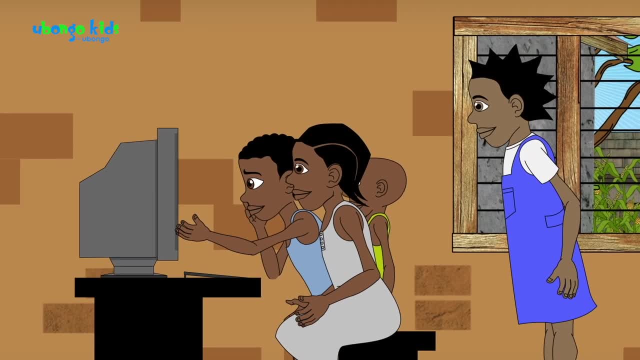 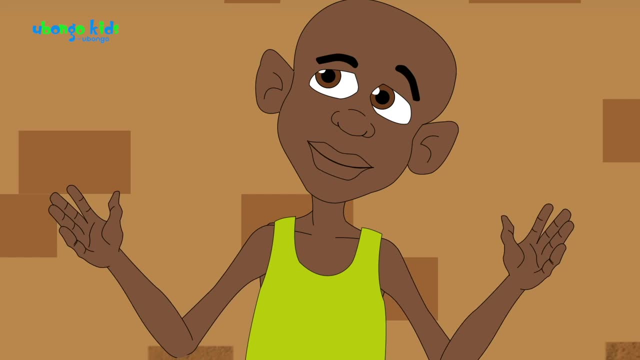 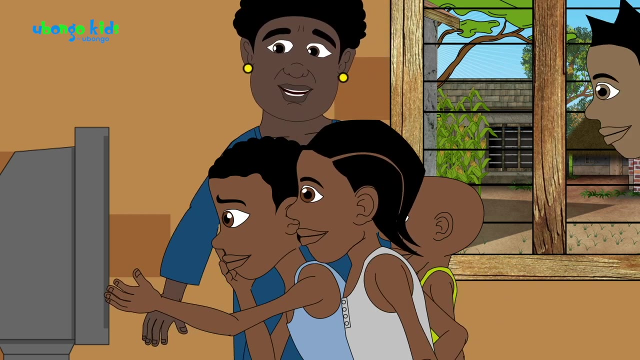 All I see is gibberish. That's crazy stuff. Let's leave it to computers. We've had enough. But who makes computers? People do, That's right, People like me and you. So who will tell computers what they should do? 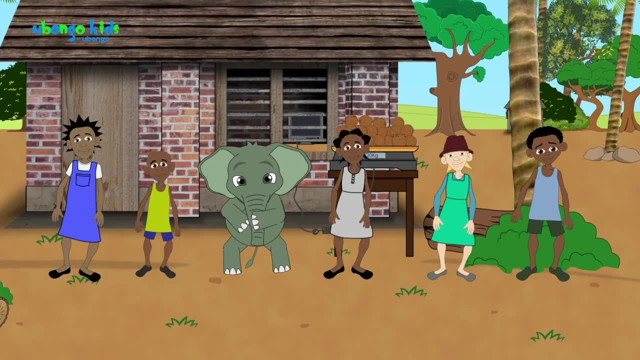 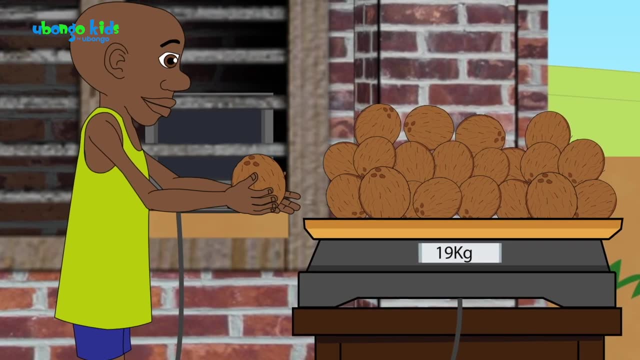 If you can code, then it's up to you. Code code, code, code, code code, Putting together commands. Code code, code, code, code code. We are creating programs When we write coding languages. 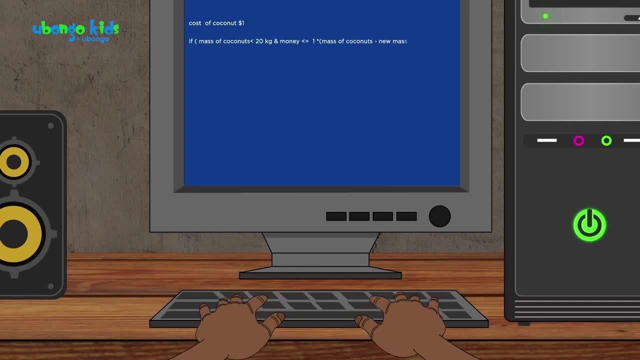 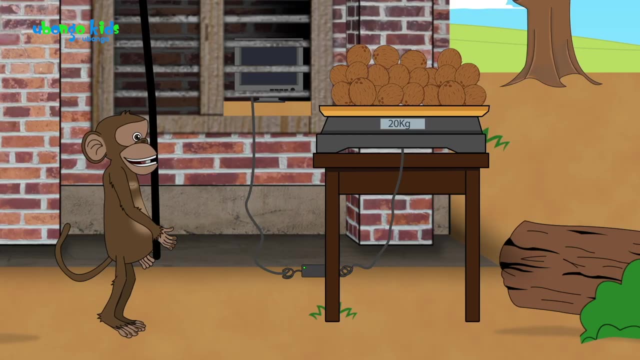 computers understand And with some practice, any of us can Code, code, code, code, code code. Putting together commands, Code, code, code, code, code, code code. We are creating programs. What's it do first? 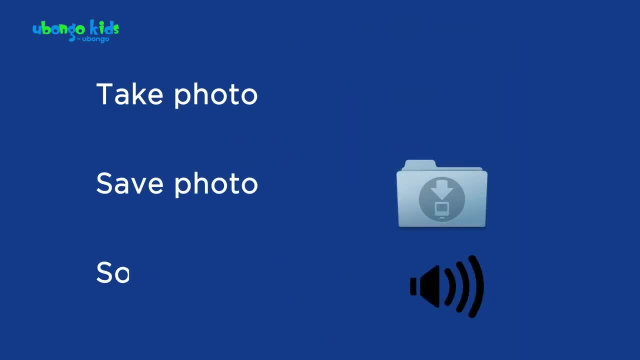 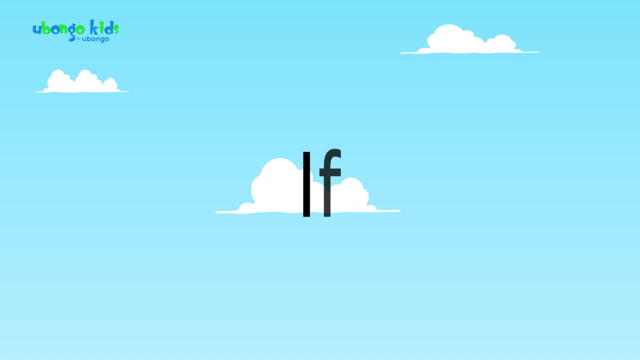 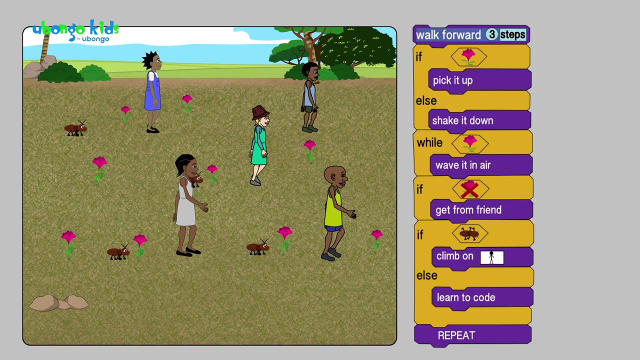 What next? in systematic steps: If and then else. if not, not, then when Let's make a code using the code, The commands if, if else else, and while while Let's code Walk forward, three steps. 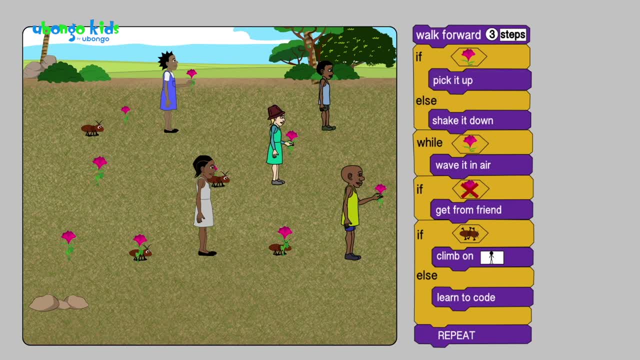 If you see a flower, pick it up. pick it up, Else shake, shake it down. shake it down. While you have a flower, wave your flower in the air. If you don't have a flower, find a friend with one flower. 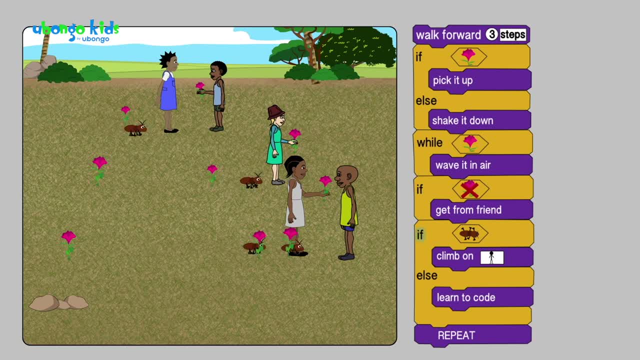 And take it, but take it fair. If you are an ant, climb up on a plant. Else, tell the ants about today's code. lesson Repeat: Walk forward three steps. If you see a flower, pick it up. pick it up. 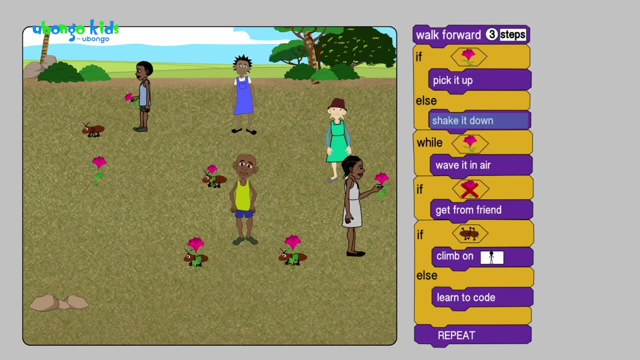 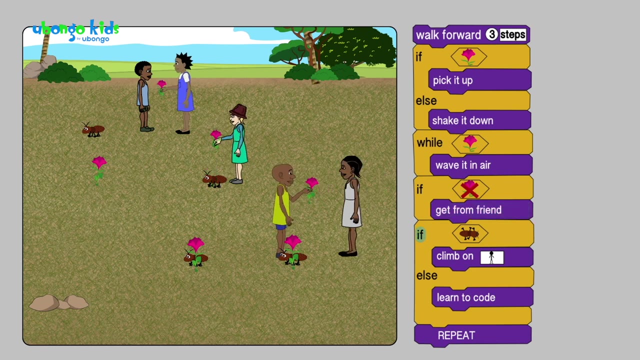 Else, shake, shake it down. shake it down While you have a flower, wave your flower in the air. If you don't have a flower, find a friend with one flower And take it, but take it fair. If you are an ant, climb up on a person. 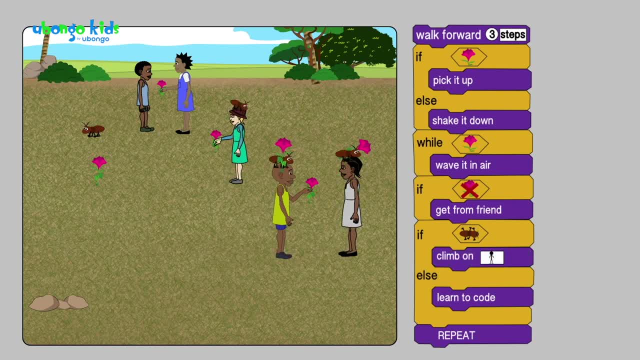 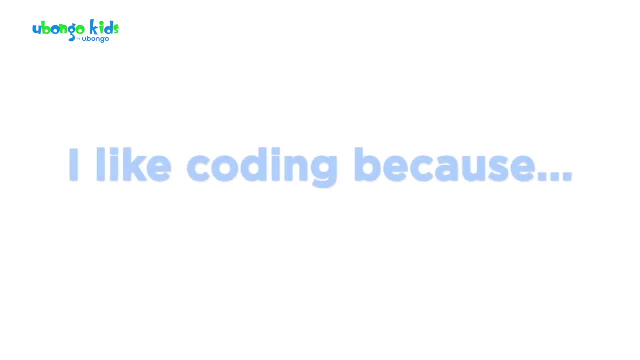 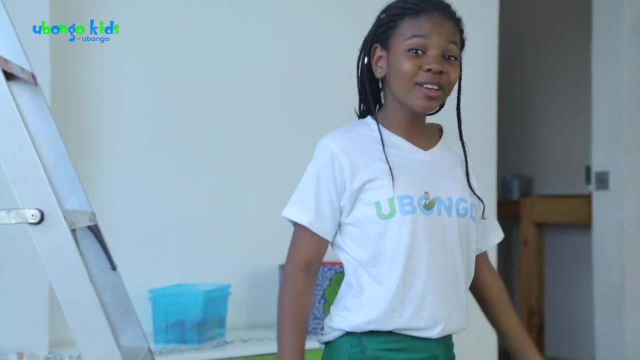 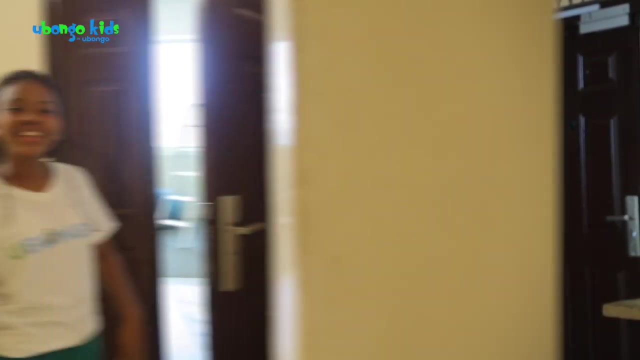 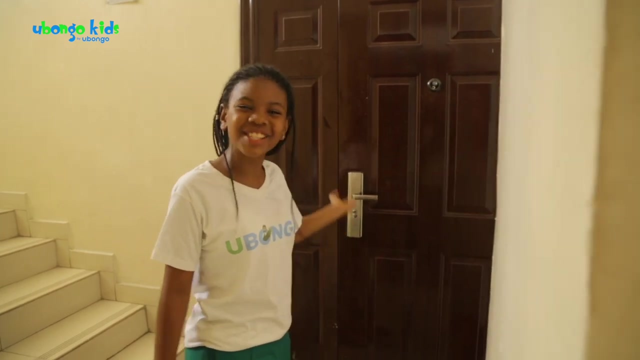 Else tell the ants about today's code lesson. Repeat about today's code lesson. I like coding because I am able to make anything out of it. Coding is everywhere around us. We use the logic of if and then every single day, But sometimes we just don't realize. Like this door. I know if I push the door then the door will close. That's code. And this fan. I know that if I press 1,. 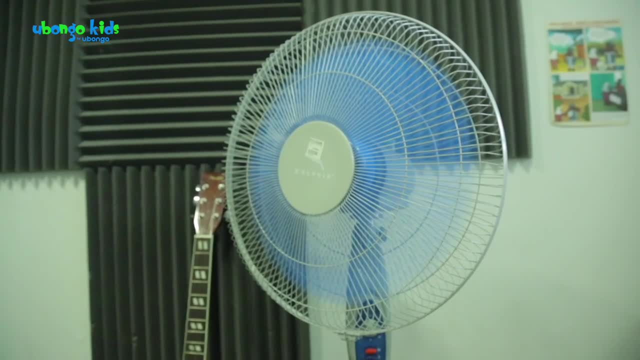 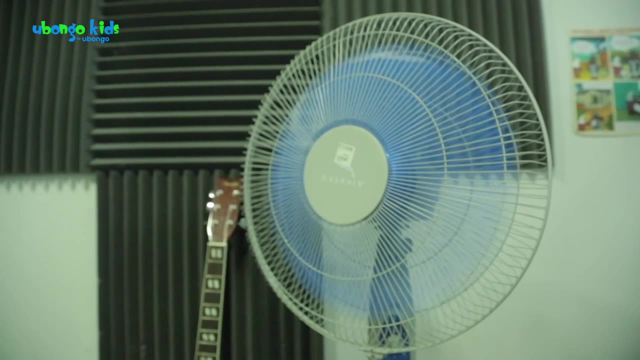 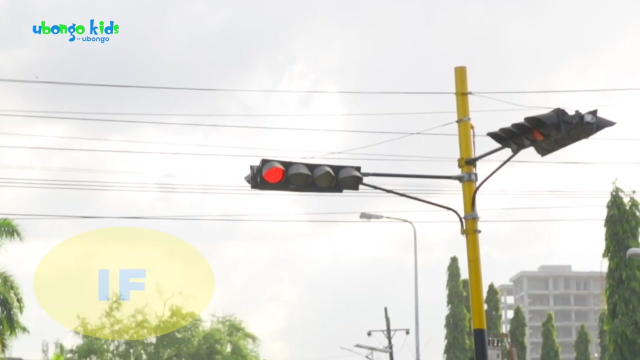 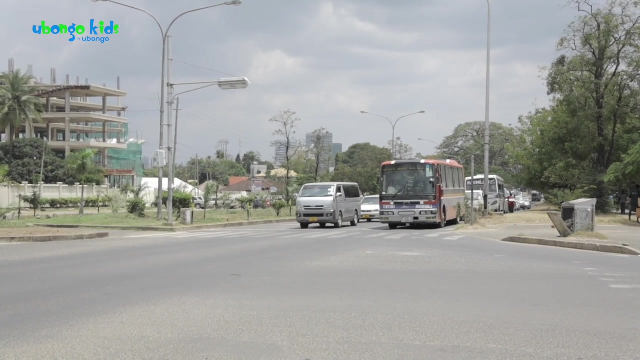 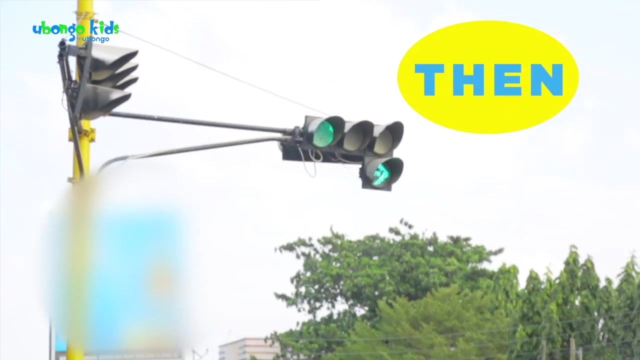 1,, Then it will spin slowly. And I know that if I press 2, then it will spin faster. That is code And traffic light. If it's red, then stop. If it's green, then go, go, go. 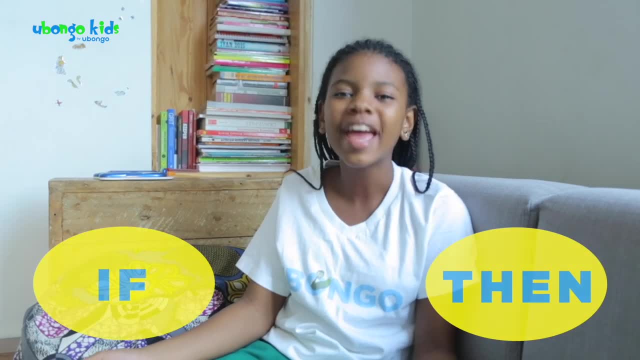 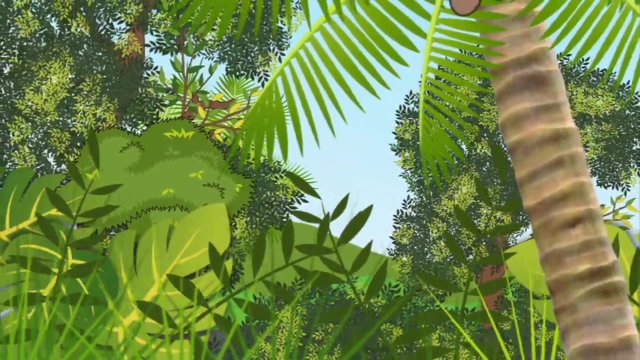 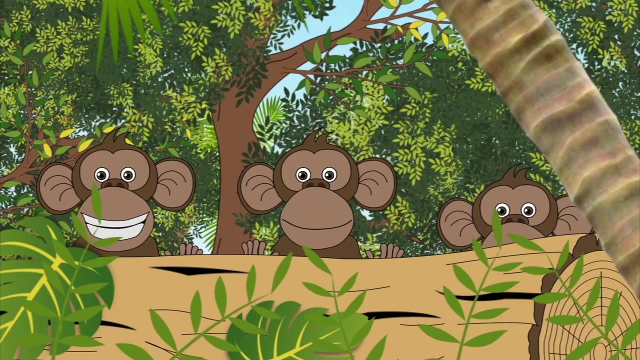 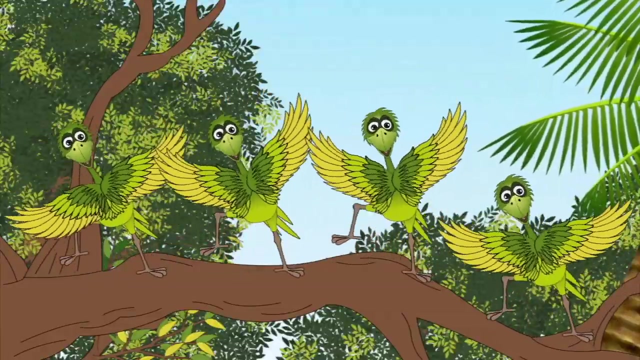 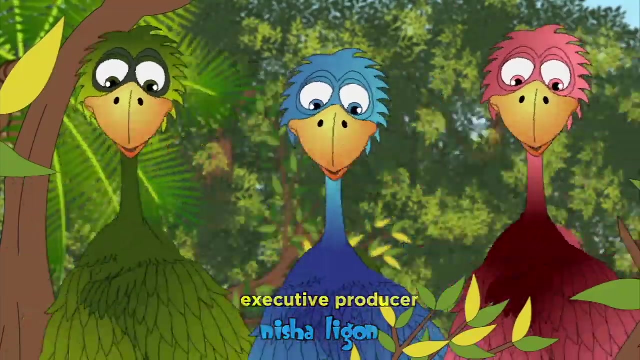 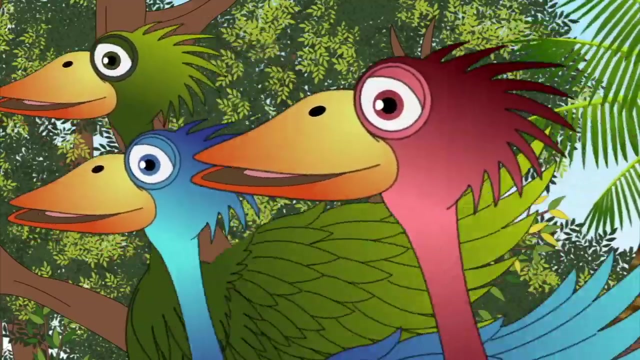 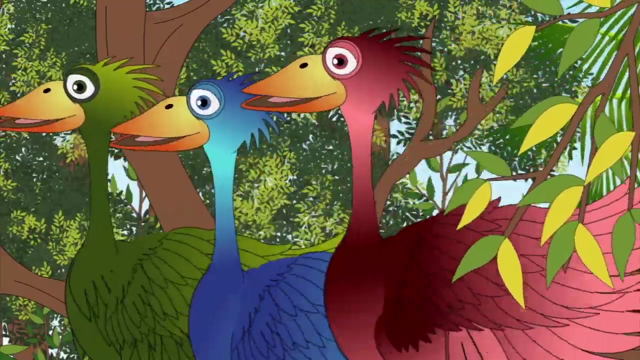 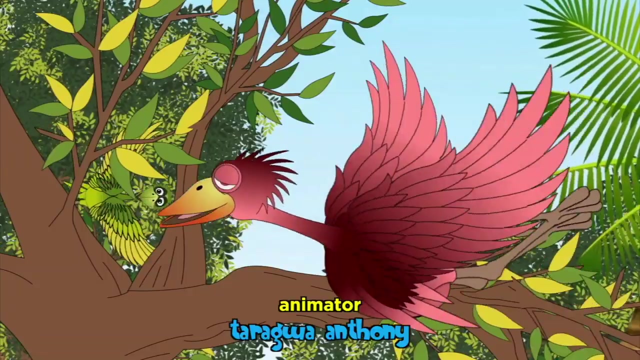 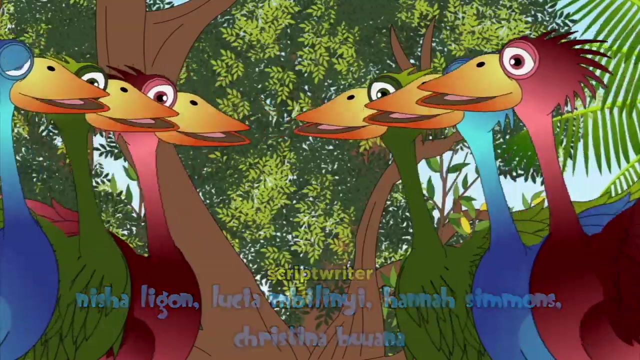 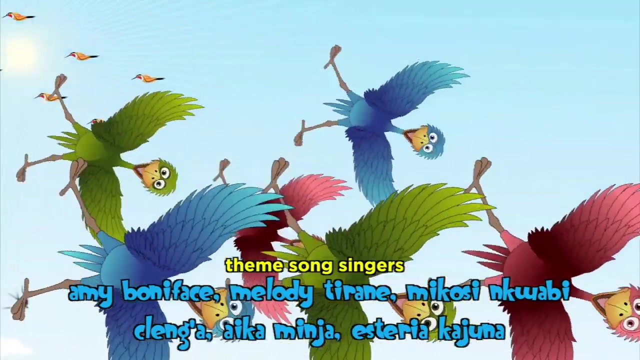 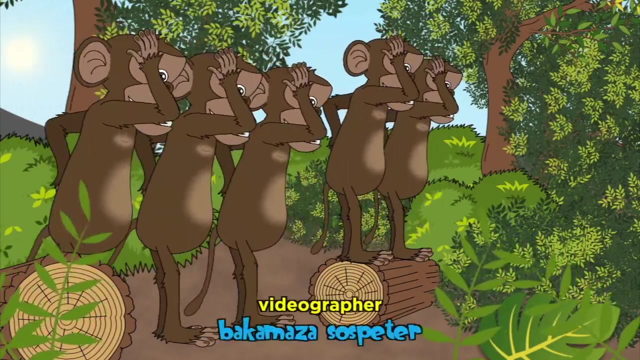 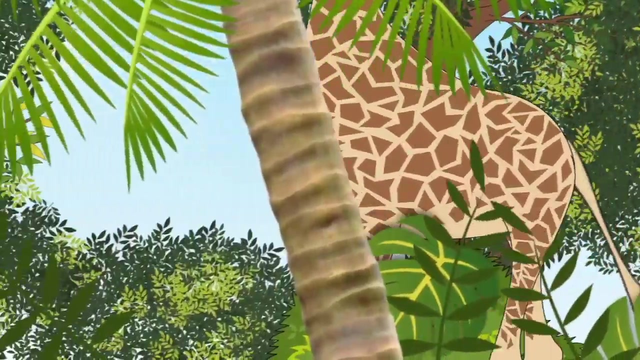 And look around you and see how you will use code in your everyday life. Mathematics, How I love it. Mathematics. Sing about the magic of mathematics, Mathematics, Making number magic with mathematics, Mathematics, Sing about the magic of mathematics, Mathematics. What is mathematics? Mental acrobatics. 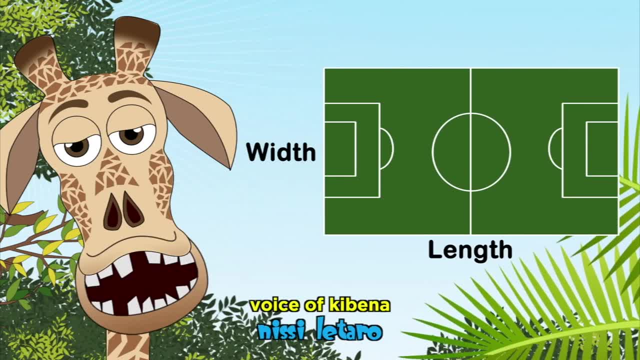 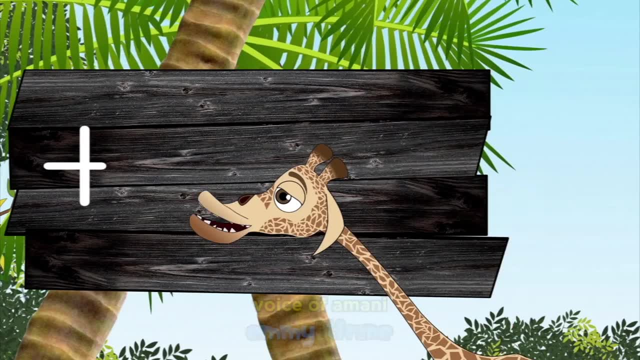 Every day, all the time. just use your mind. You use math when you measure, Read, learn, learn Solving problems using mental strength. Use number operations like multiplication. The number you will find is like magic from your mind. Math is a part of everyday life. 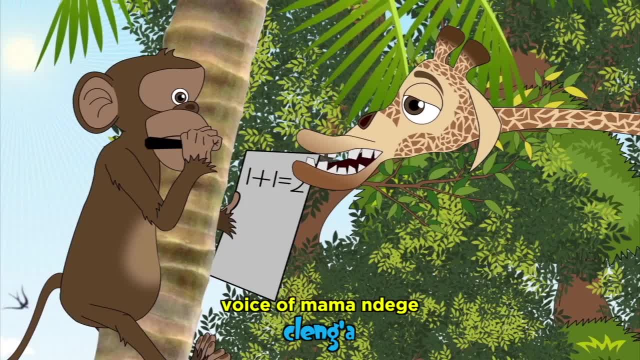 Just add subtract, divide and multiply, Can you solve the problem? Did you get the answer? Just use your brain and you can do it. sir, Now don't you rush it, Just take it slow. You must be careful. 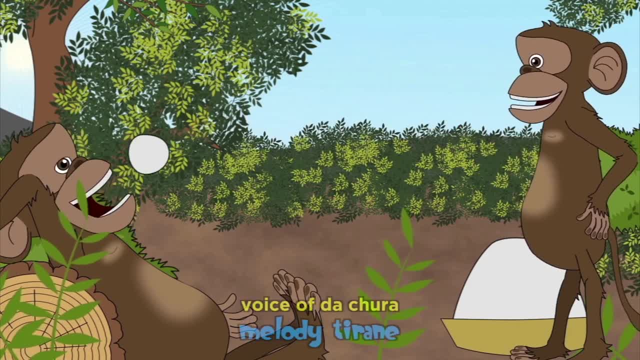 Don't you know? You use math for all things in life. When you eat ugali, you count your bites In a parade. count the steps you take. Just listen when I rap, I'm using math. Calculate the distance when you drive your car. 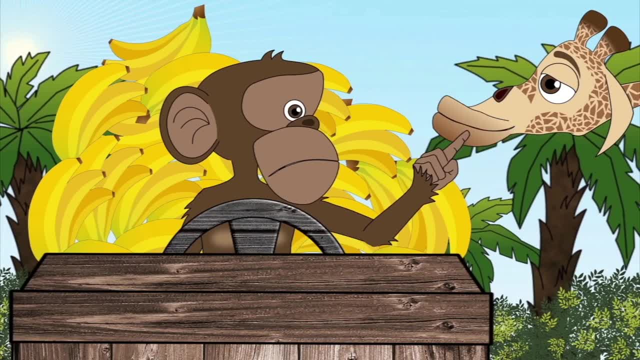 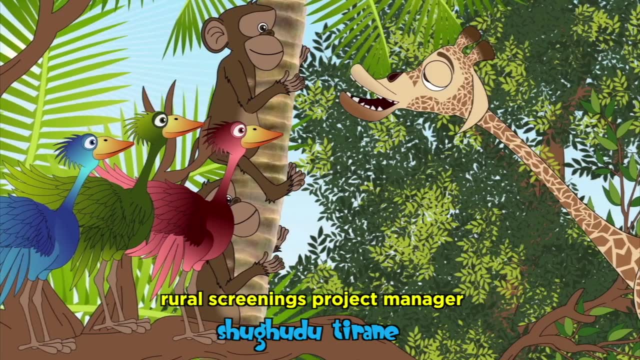 So you will know if you have gone far. Here's something else for you to count. Can you count the teeth in my mouth? We can measure width, length and depth And represent with X, Y and Z. Math is used for everything. 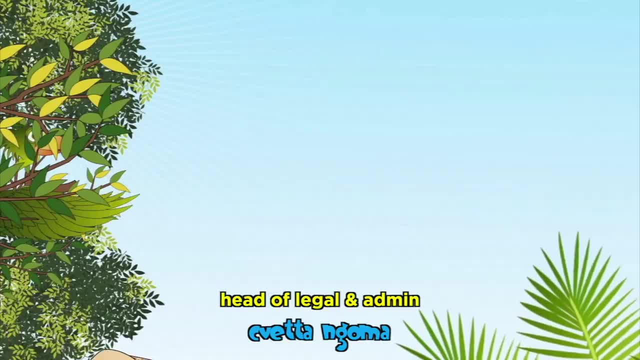 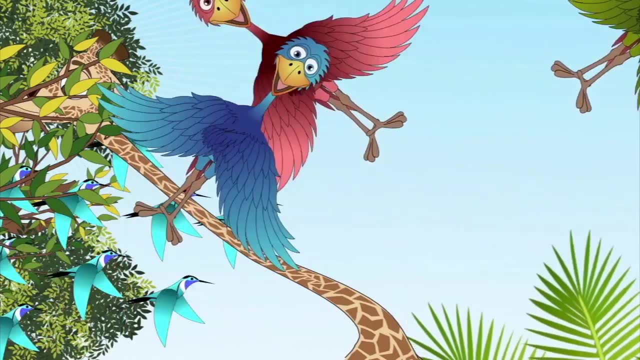 Just do the numbers in your head Now. try to add up all the numbers. Sports on my neck, How many do you see? And I even use math to get leaves off the tree. Mathematics, mathematics. You understand now, right. 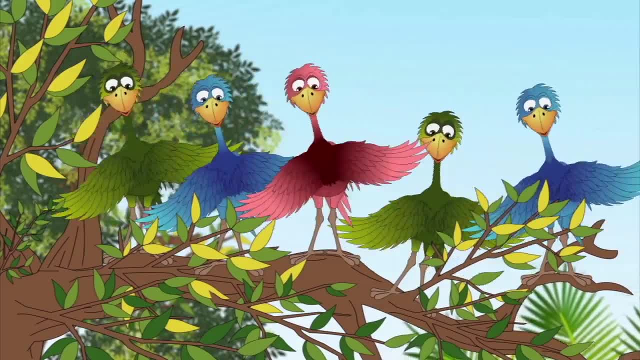 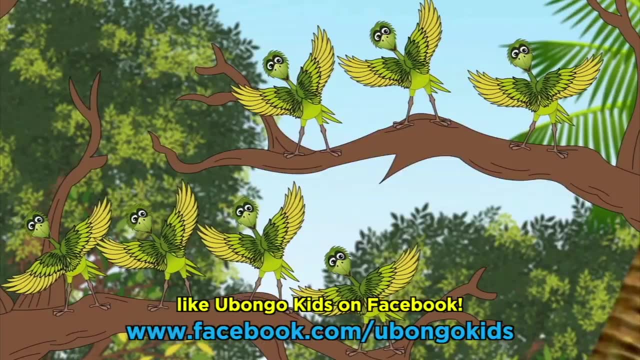 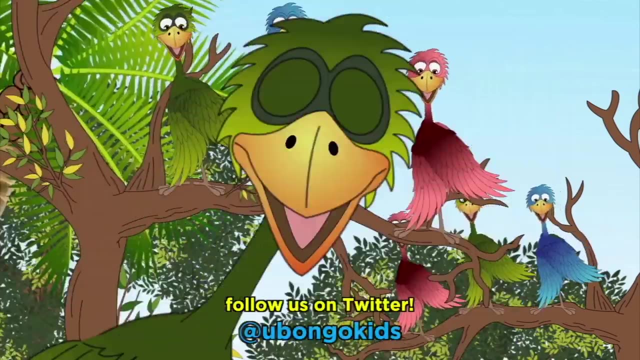 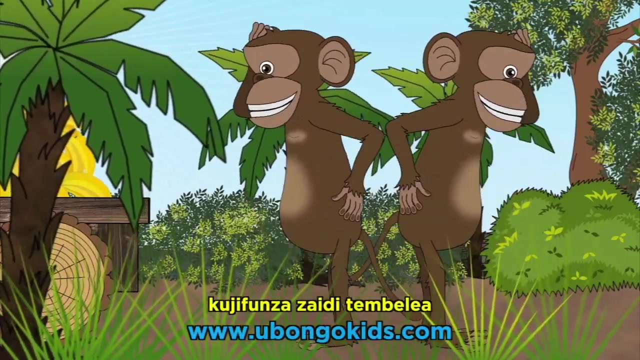 Mathematics, yeah, yeah, Okay, Mathematics, how I love it. Mathematics, yeah, yeah, Sing about the magic of mathematics, Mathematics, yeah, yeah, Making numbers Magic with mathematics, Mathematics, yeah, yeah, Yeah, yeah.